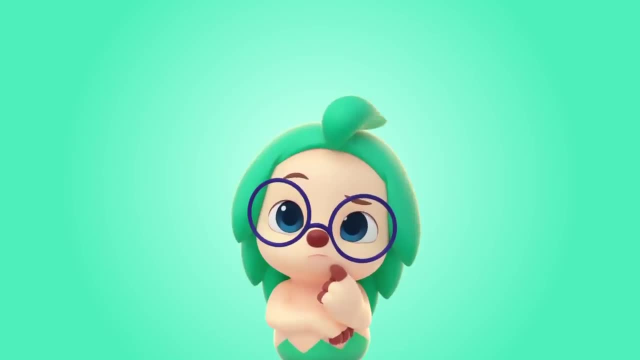 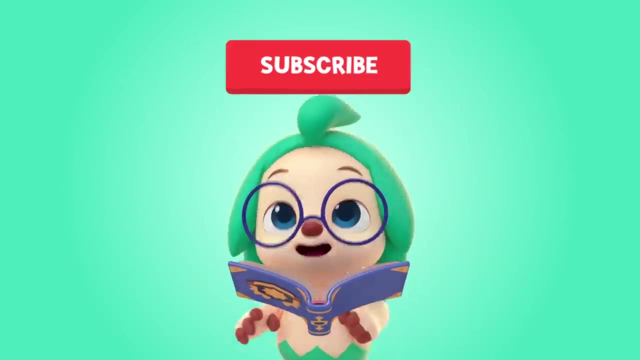 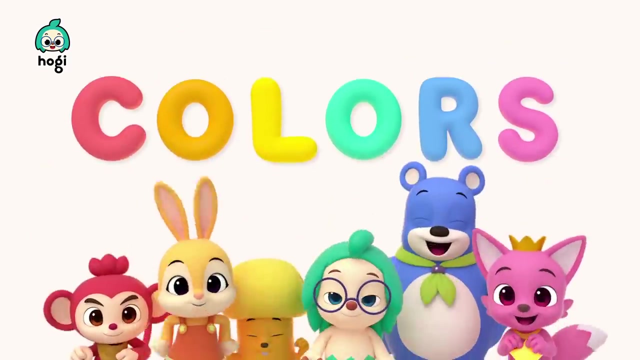 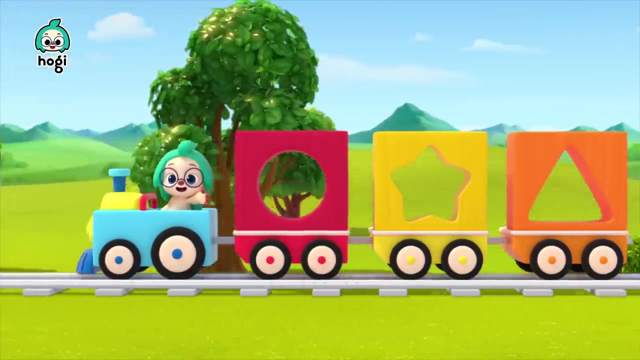 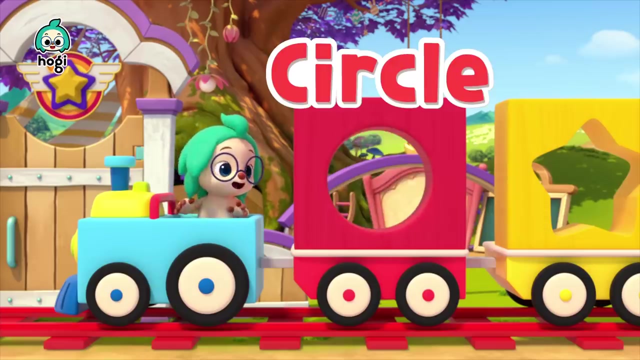 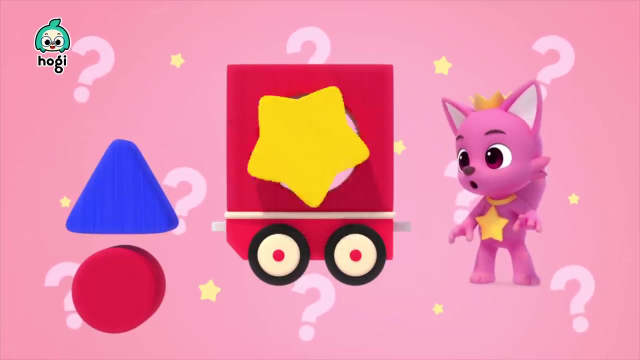 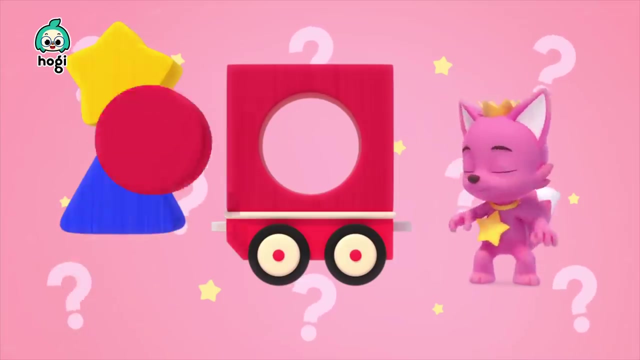 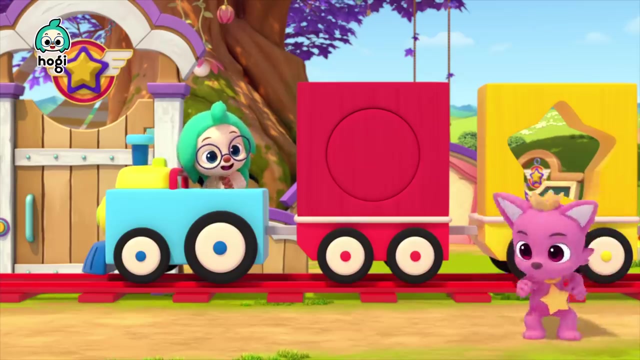 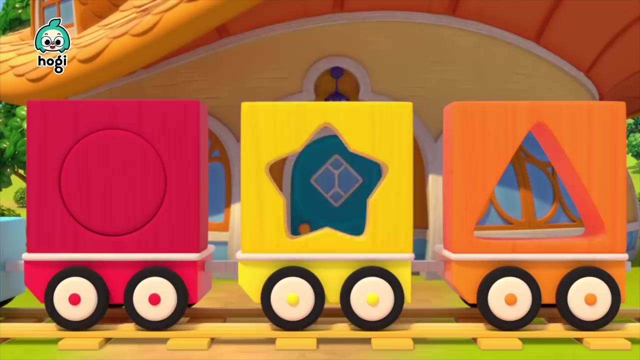 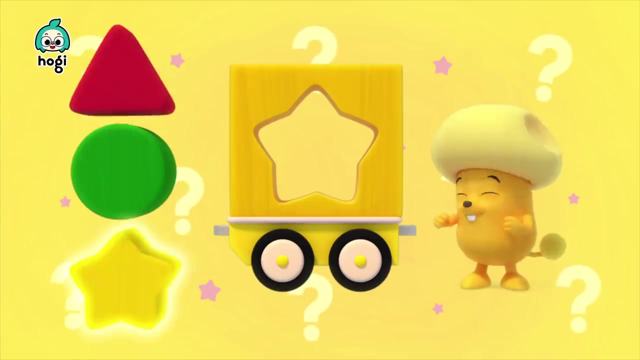 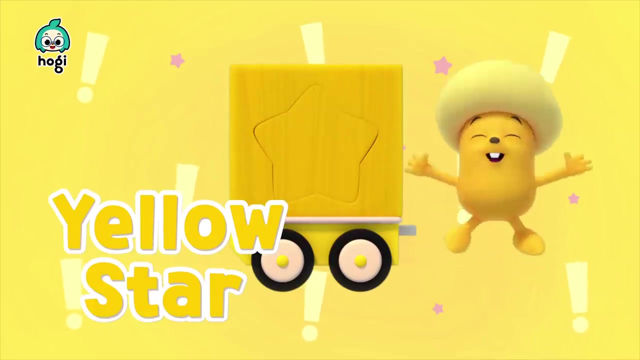 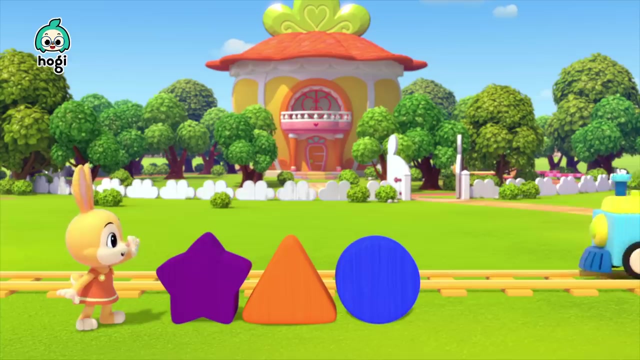 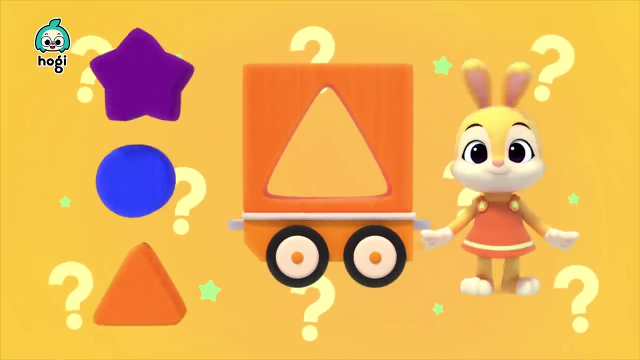 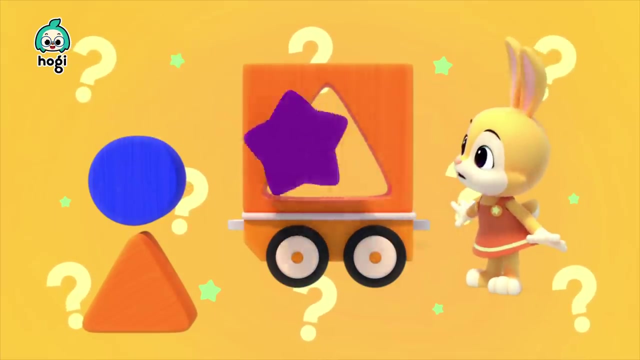 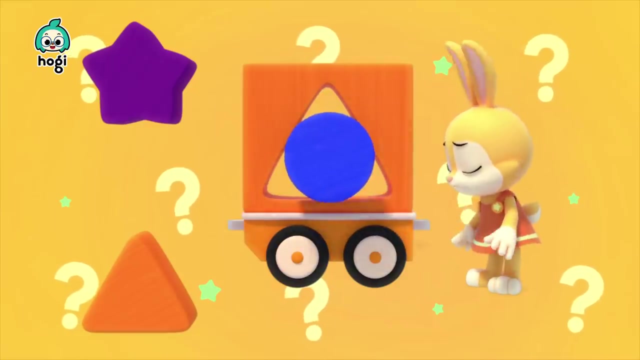 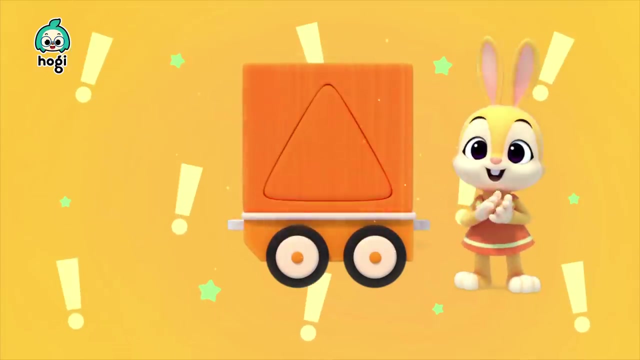 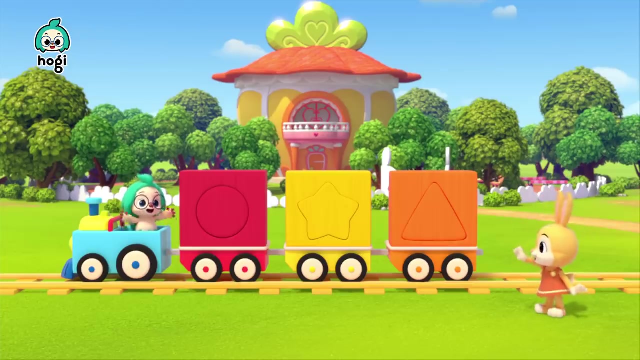 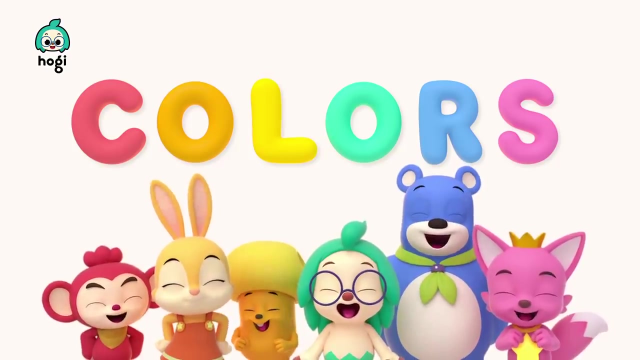 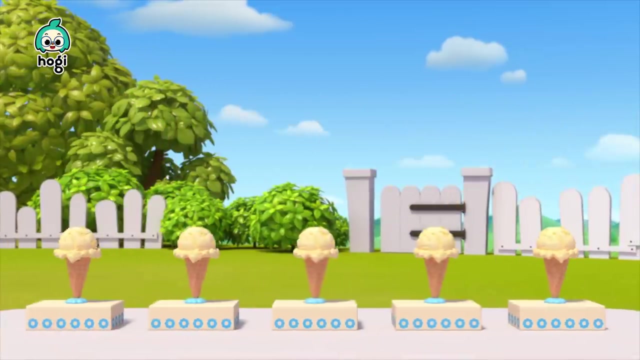 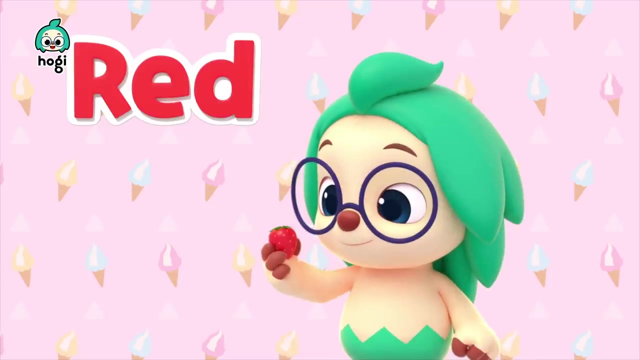 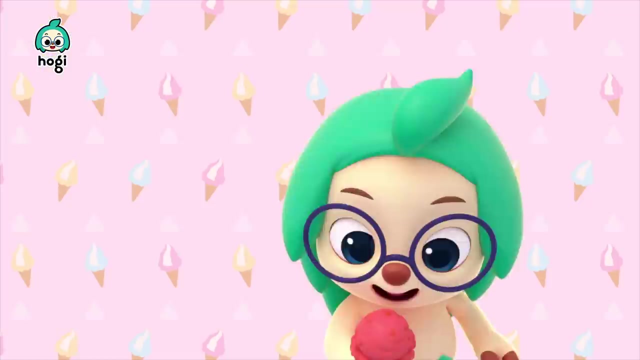 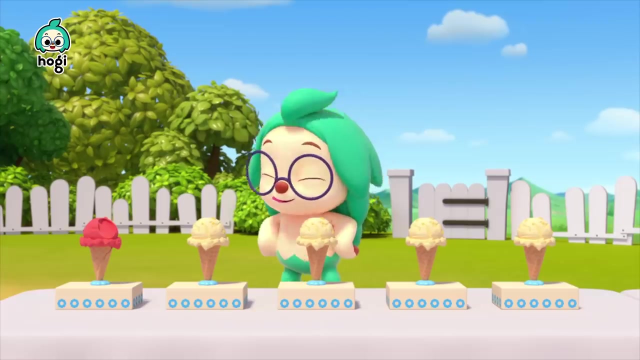 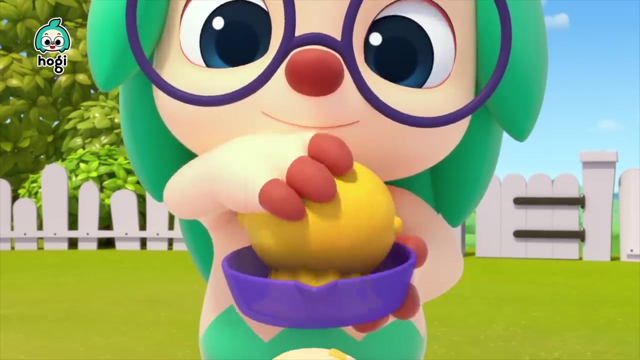 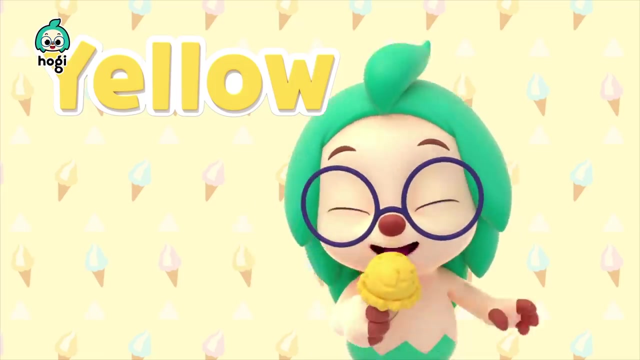 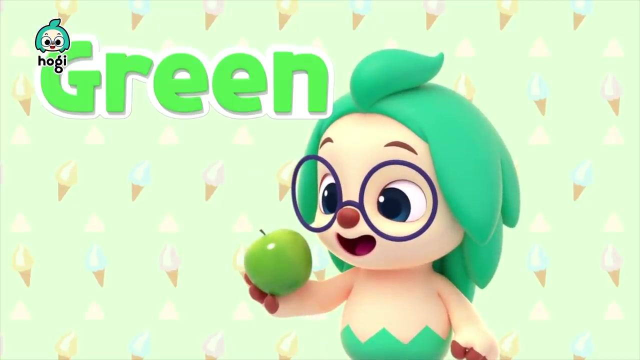 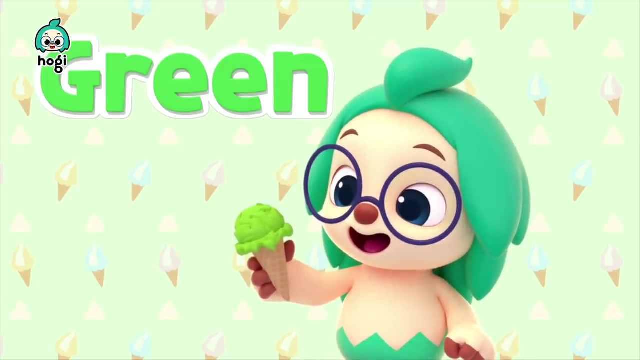 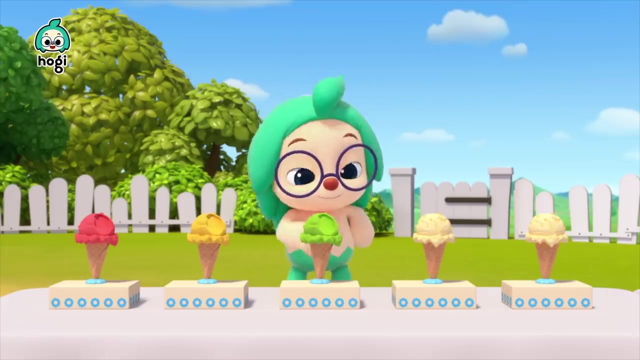 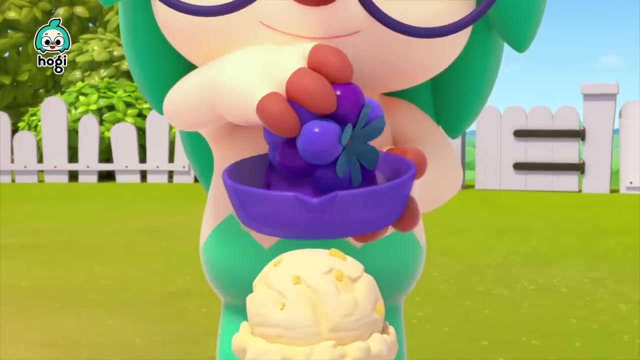 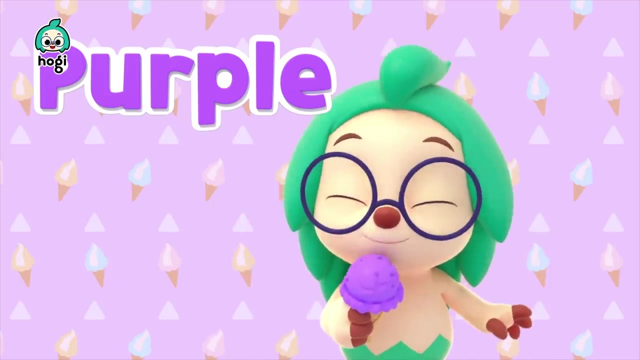 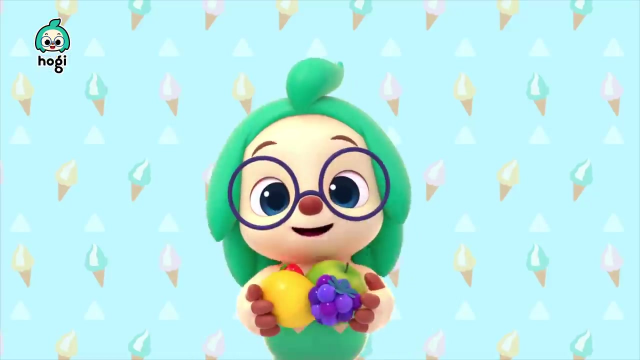 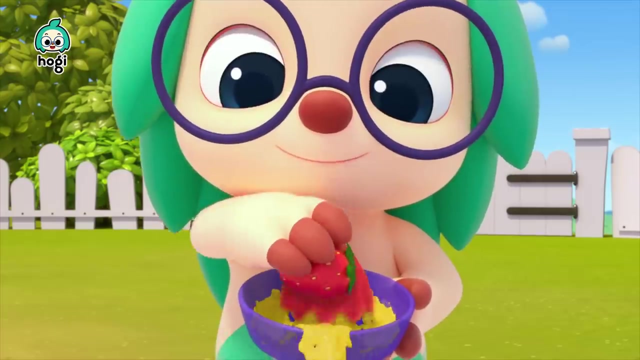 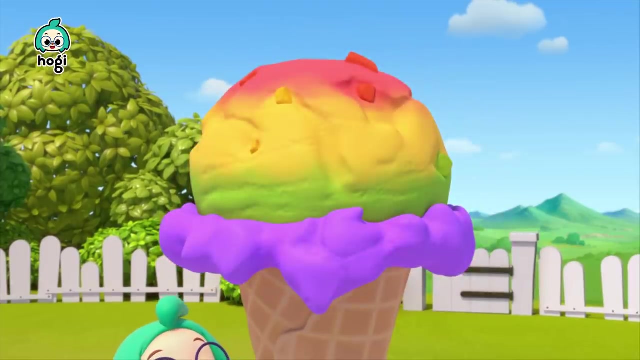 Pinkfong, Subscribe and like Hoggie. Colors Circle: Red circle, Blue circle, Star, Yellow, star Triangle, Orange triangle, Orange triangle. Colors Red circle: Red, Red, Yellow, Yellow, Green, Green, Purple, Red, Yellow, Green, Purple, Red, Yellow, Green, Blue, Red, Rainbow, Rainbow, Red, Blue, Red, Blue, Red, Blue. 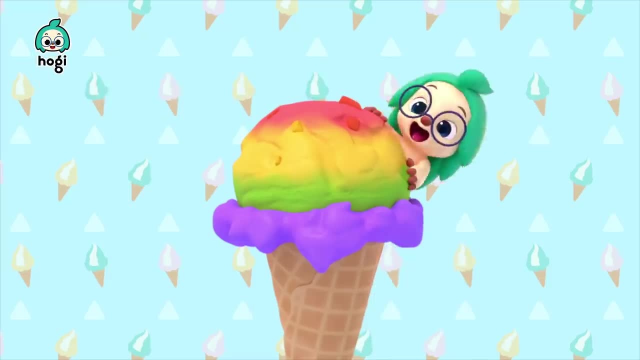 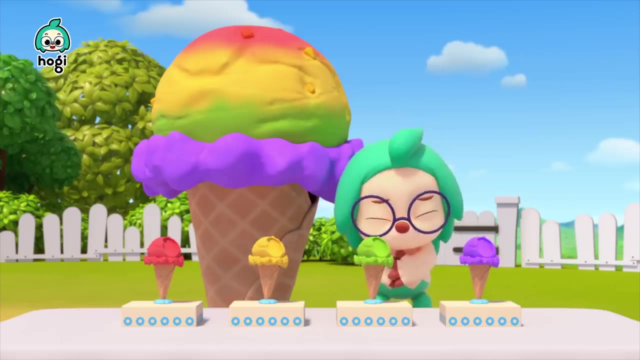 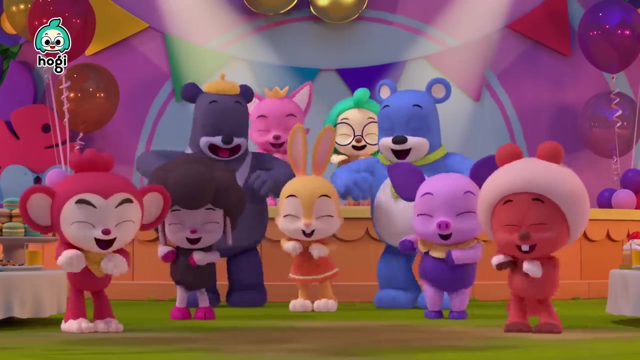 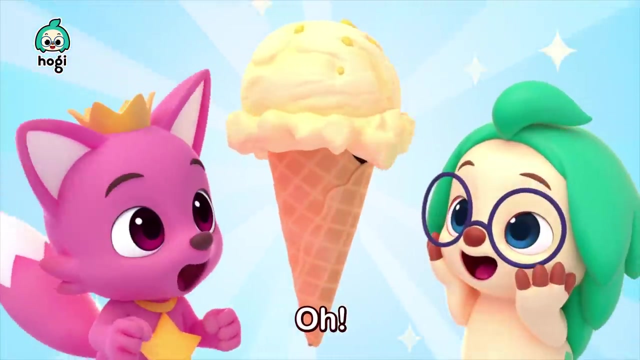 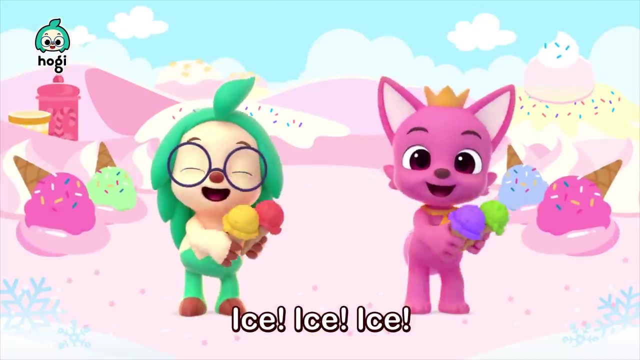 Blue, Red, Blue, Red, Blue, Blue, Blue, Blue, Blue Blue, Pinkfong, Pinkfong, Pinkfong. Ice, ice ice cream. Yummy, yummy, and my tummy Ice cream ha. Ice, ice, ice ice cream. Are you ready to scream for ice cream? 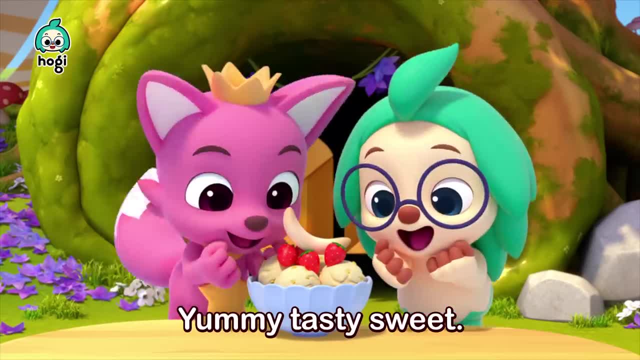 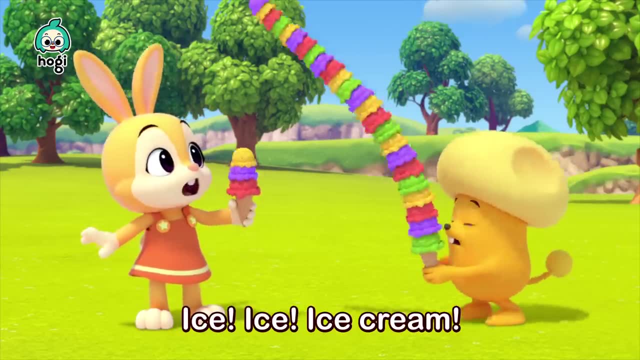 Yay, Yum yum, yummy, tasty, sweet Tom tom tummy goes party. This is my favorite treat: Ice, ice, ice cream When the day is hot and steamy, Ice cream ha, If you're happy and you know it. 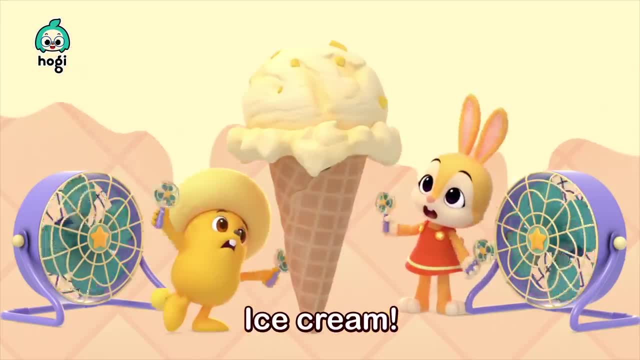 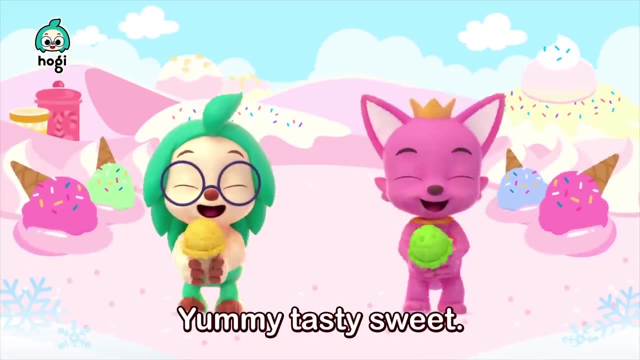 Ice cream. ha, Don't let it melt away, wake it up, Ice cream. Are you ready to scream for ice cream? Yay, Yum, yum, yummy, tasty, sweet Tom tom. tummy goes party. This is my favorite treat. 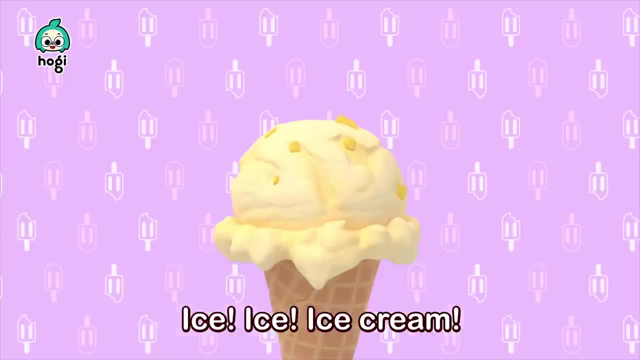 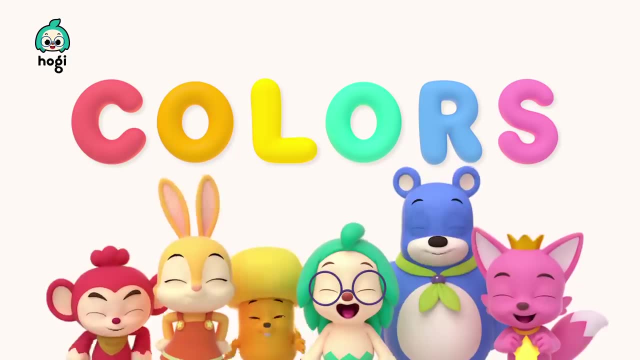 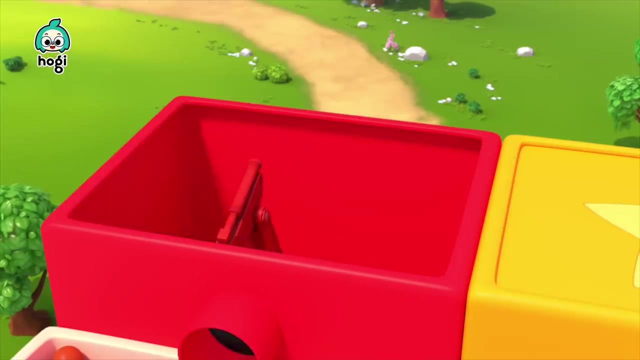 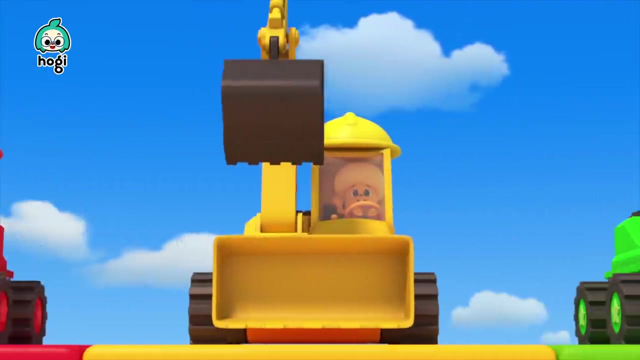 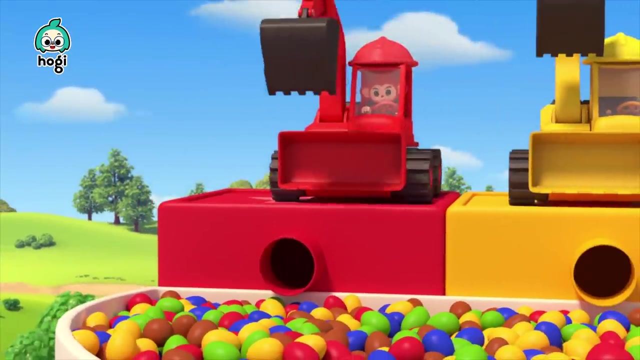 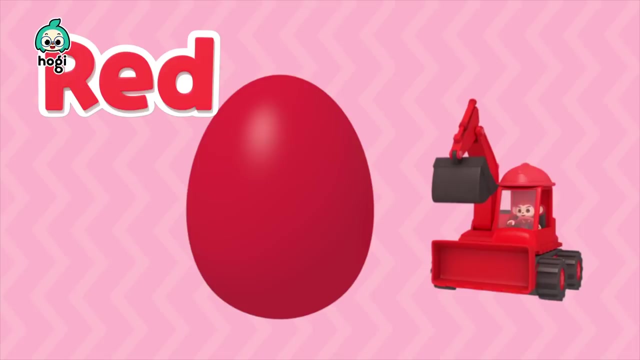 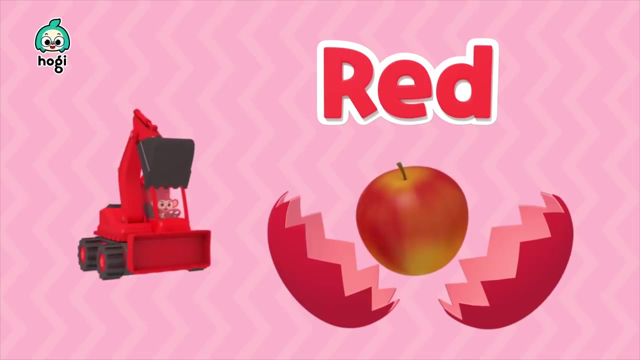 Ice, ice, ice cream. Can I have more ice cream Colors? Ha ha Ooh, Ha ha. ha. Ha ha, hi Ha ha ha, Red, Red, Yay Ha ha. 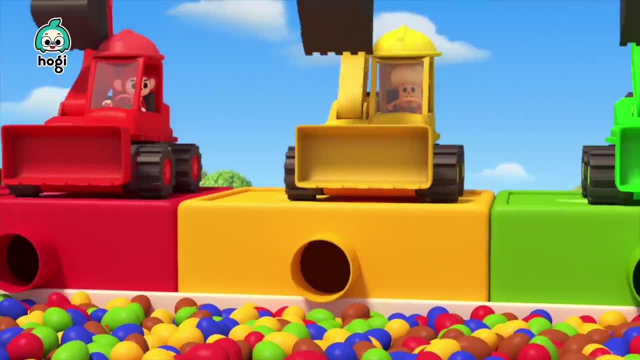 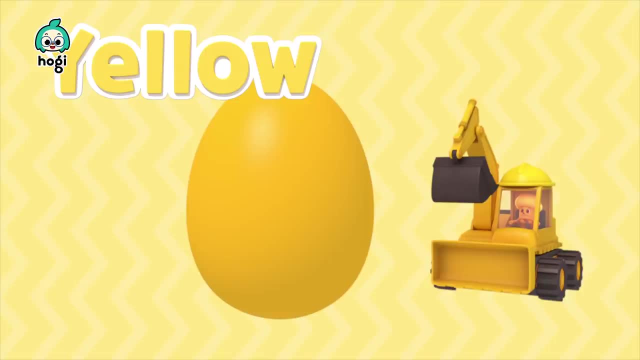 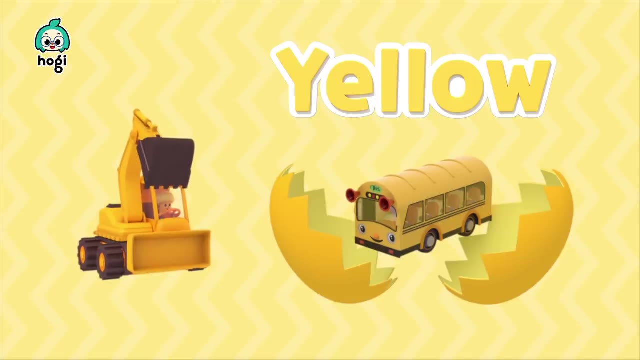 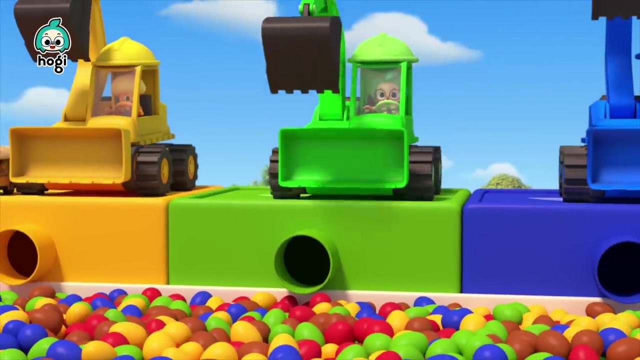 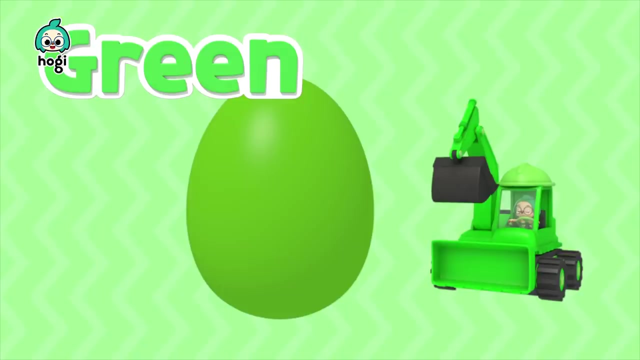 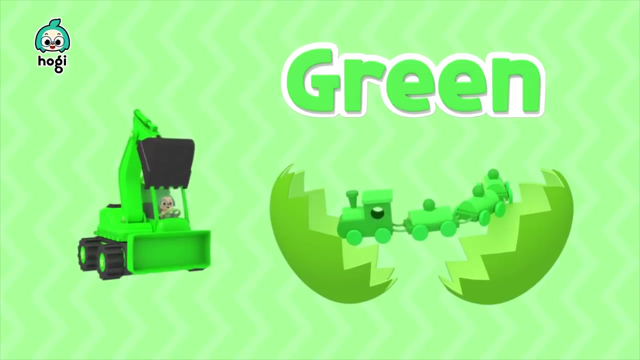 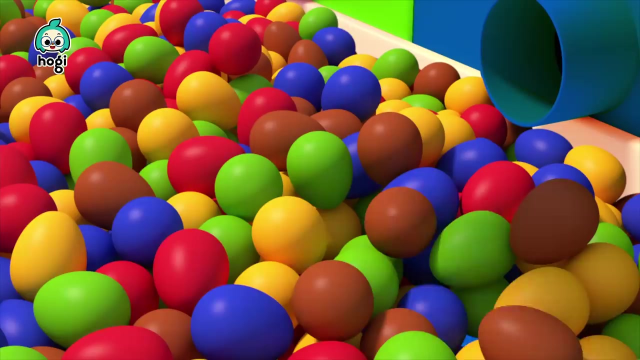 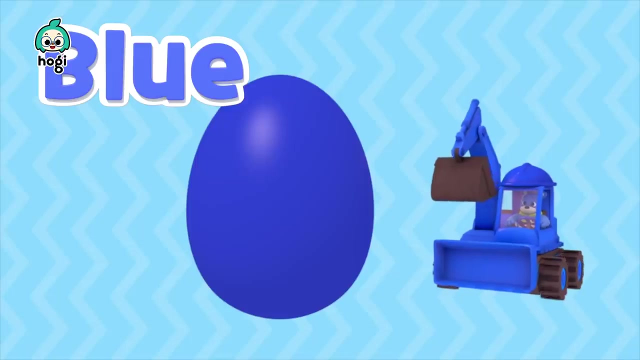 Yellow Yellow: Wow Ha ha Ha ha. Yellow Yellow, Green, Green, Yay Ha ha ha. yeah, Blue Ha ha. Blue Ha ha ha, Ha ha. 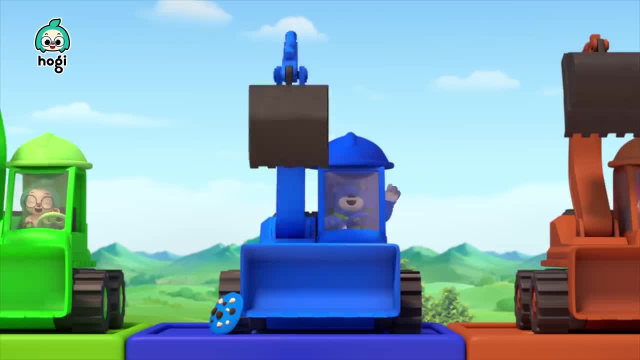 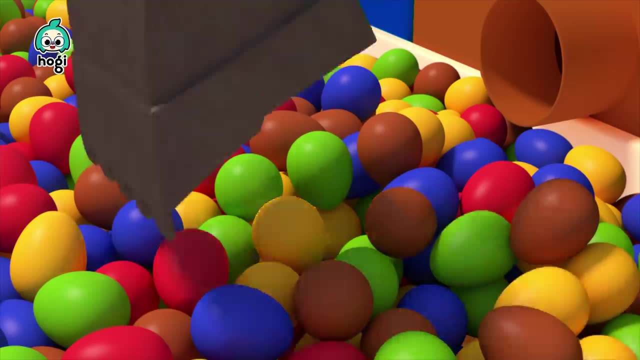 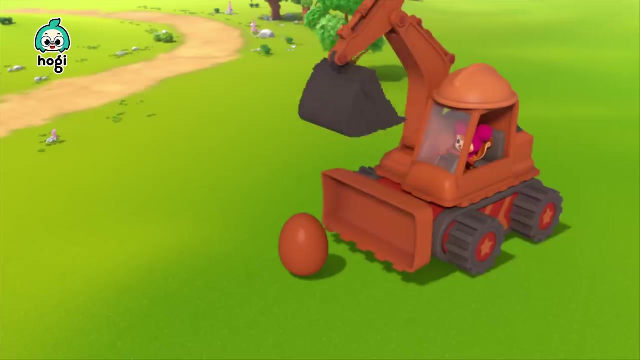 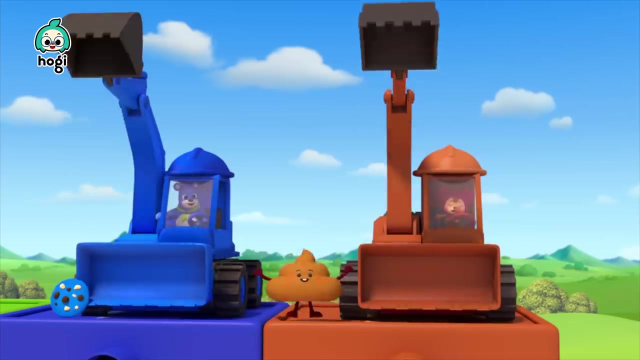 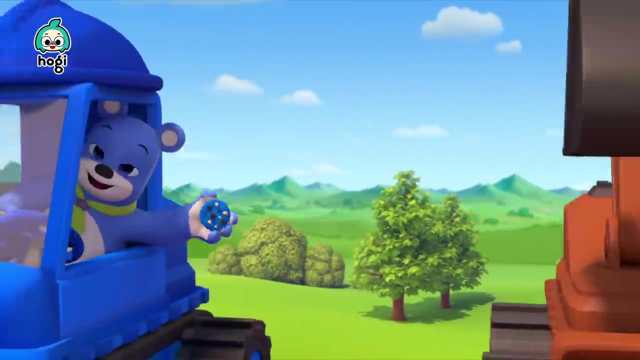 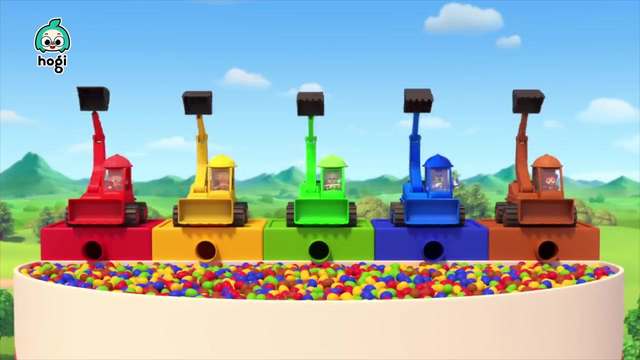 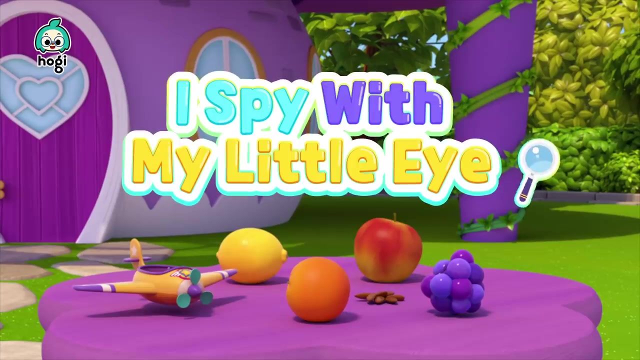 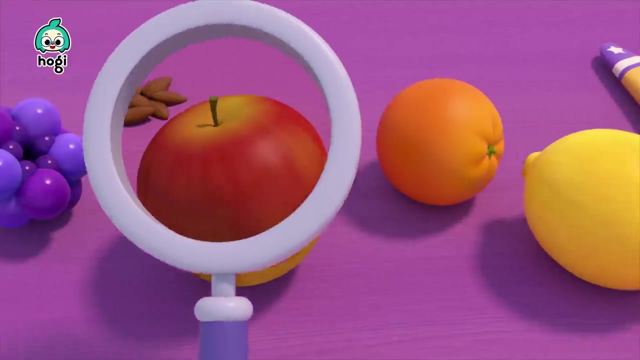 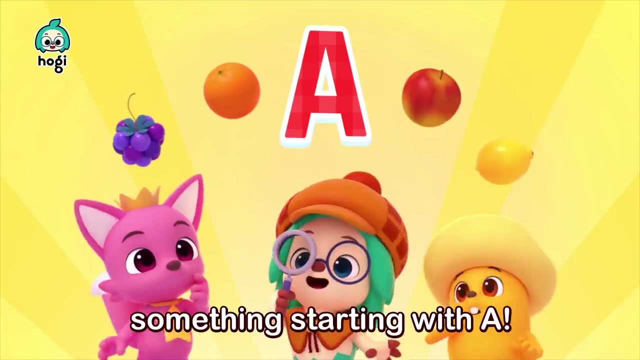 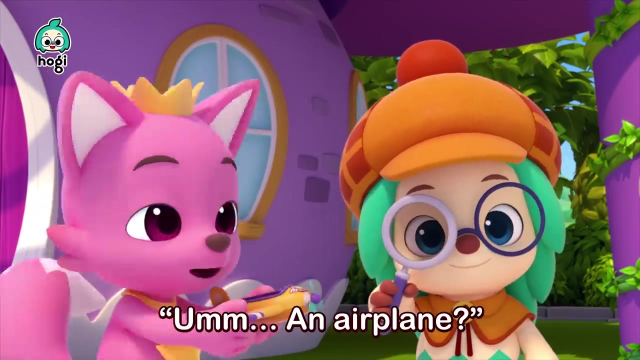 Ha ha. Green, Blue, Brown, Brown, Yeah Whoa. Sing along with Pinkfong and Hoagie. I spy with my little eye Something starting with A. I spy with my little eye Guess what it is: An airplane. 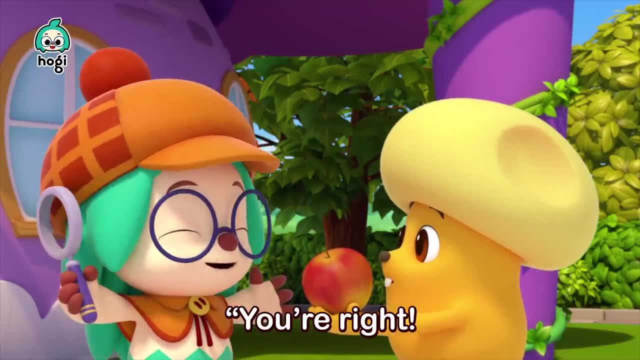 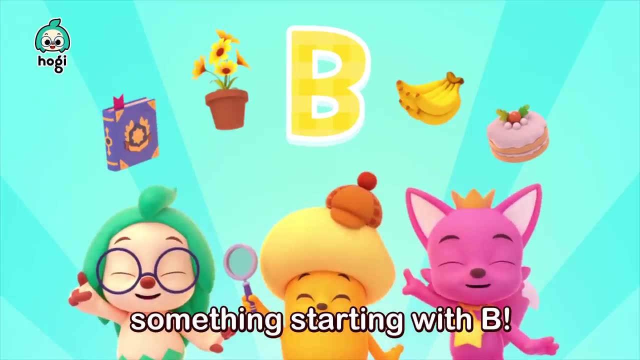 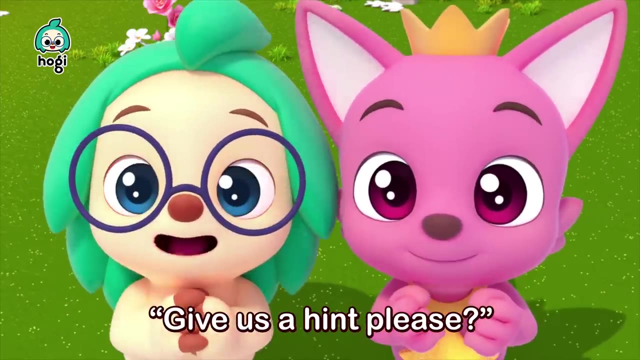 Wrong An apple. You're right, You be the spy. I spy with my little eye Something starting with E. I spy with my little eye. Guess what it is. Give us a hint, please. It is long and sweet Banana. 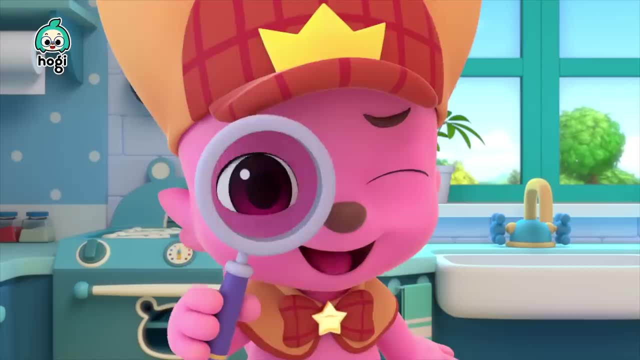 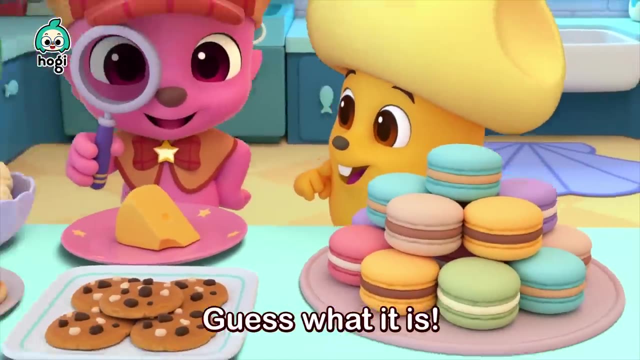 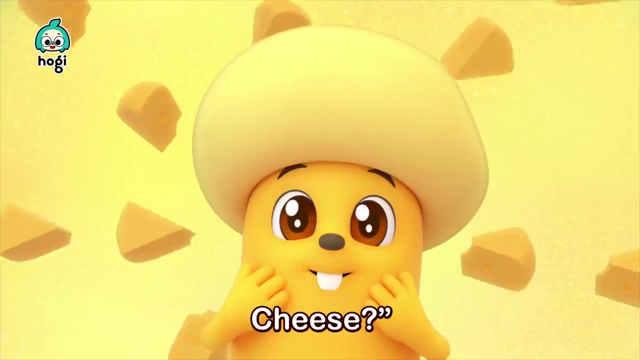 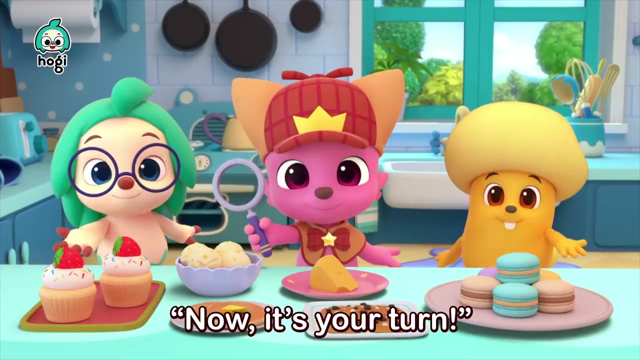 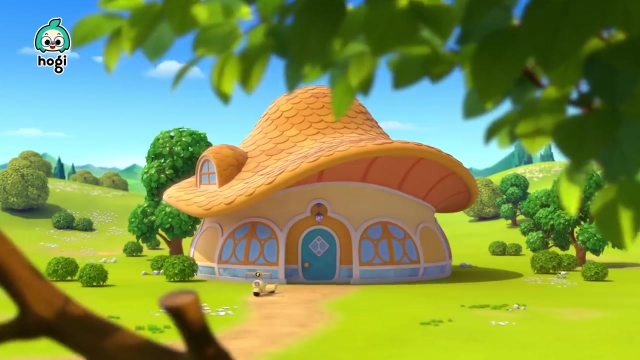 Right, Yes, Now it's your turn. I spy with my little eye Something starting with Z. I spy with my little eye. Guess what it is. Let me see. Is it Cheese? Yes, Now it's your turn. I spy with my little eye. 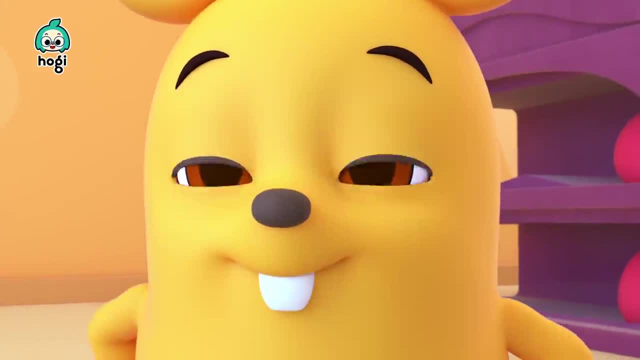 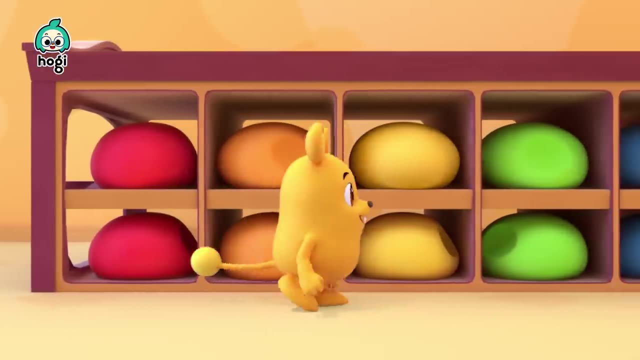 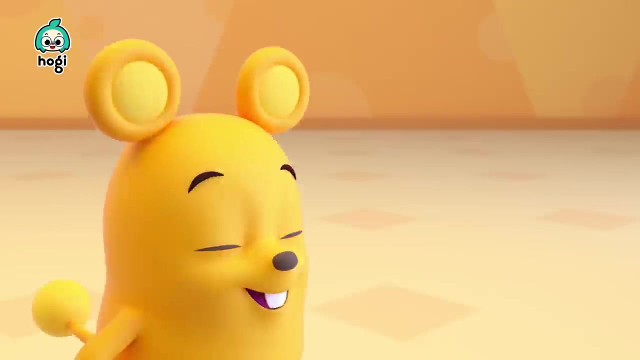 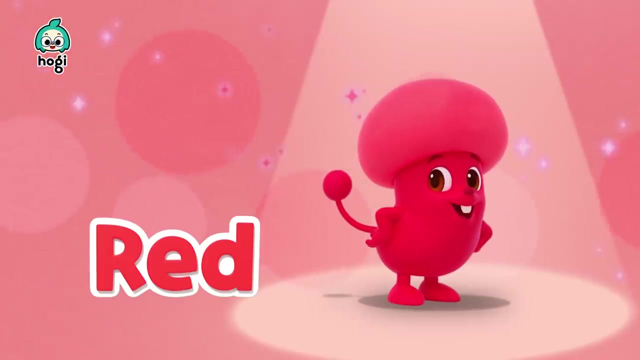 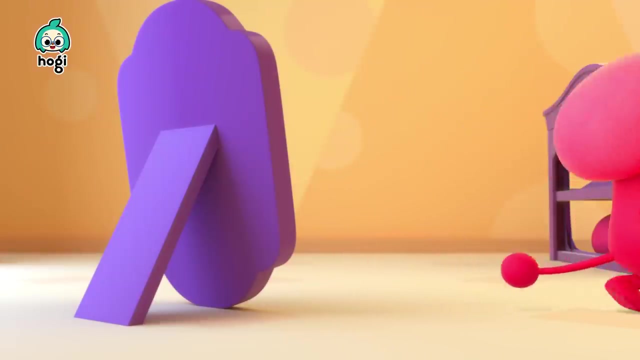 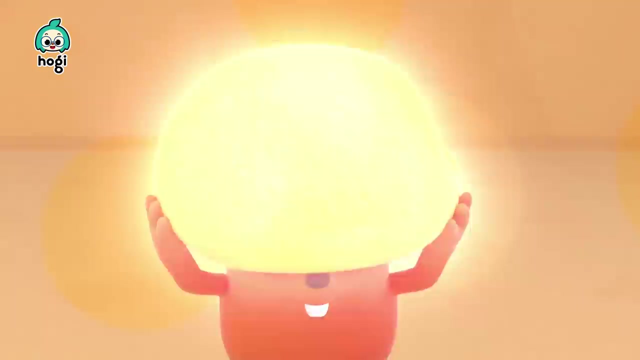 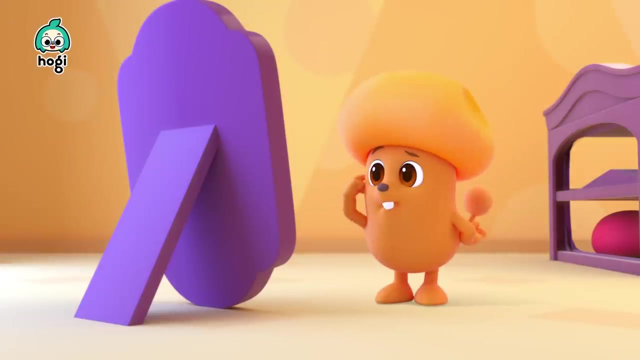 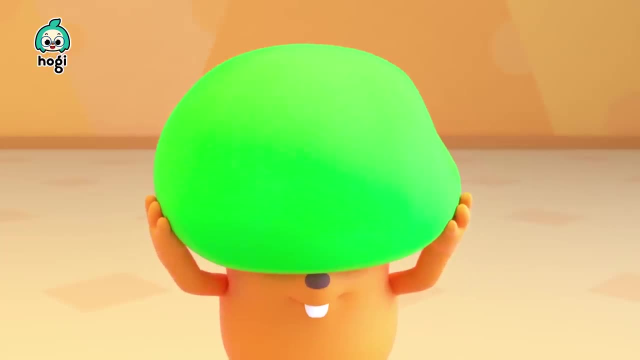 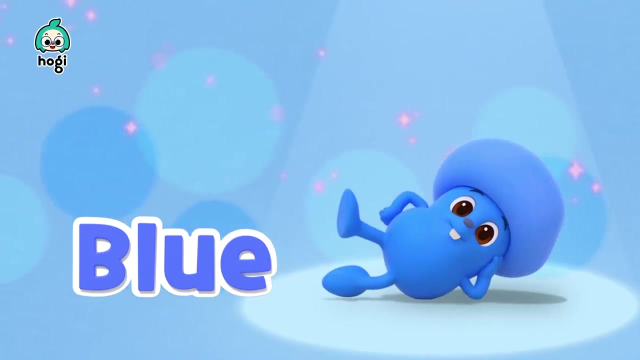 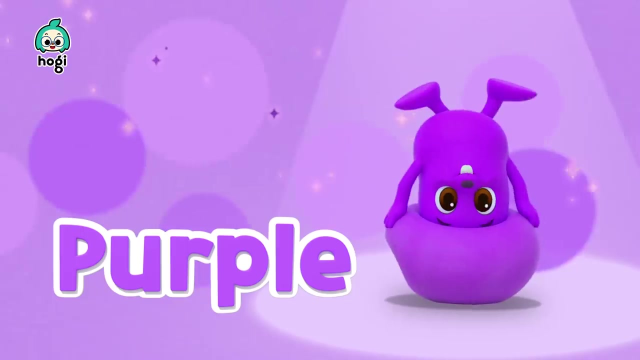 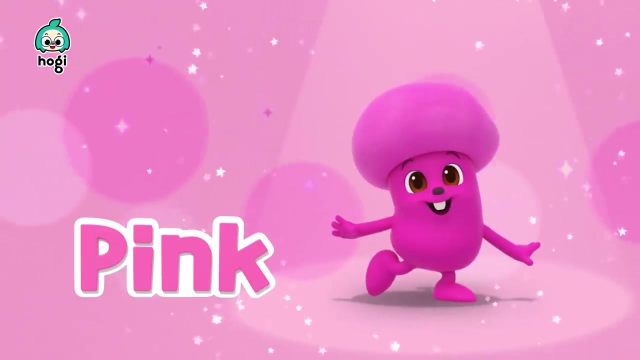 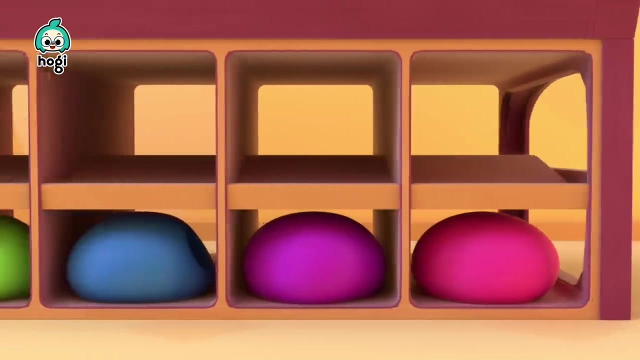 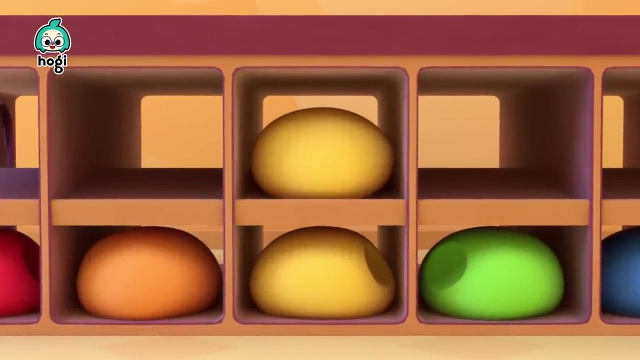 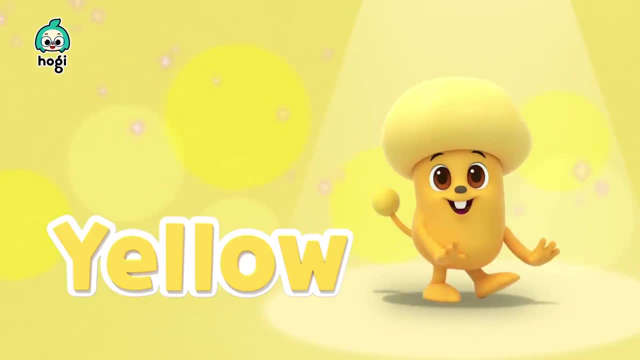 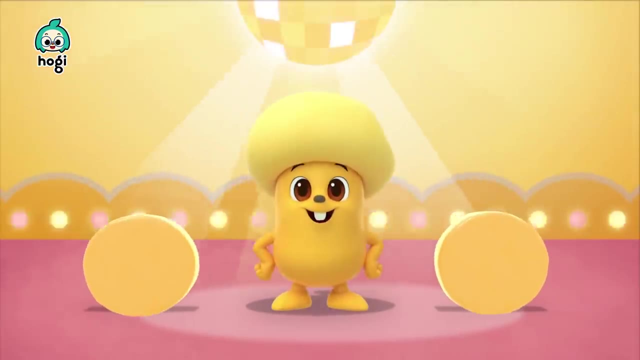 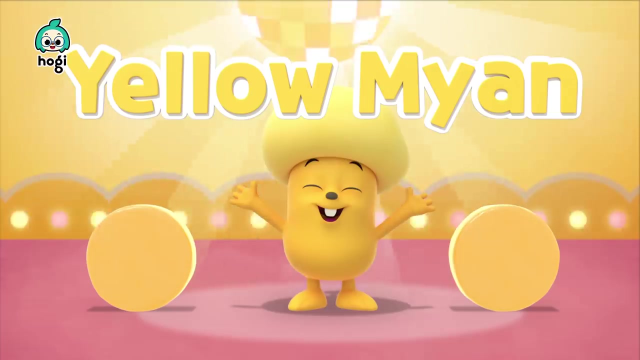 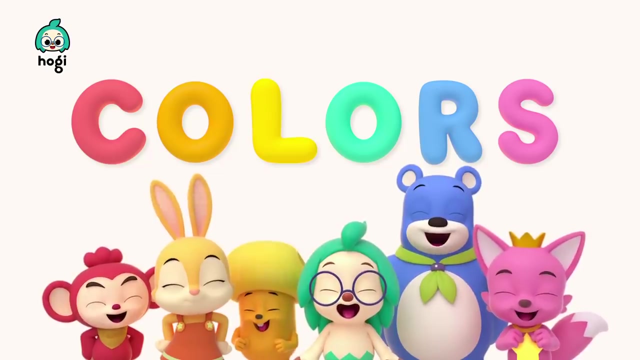 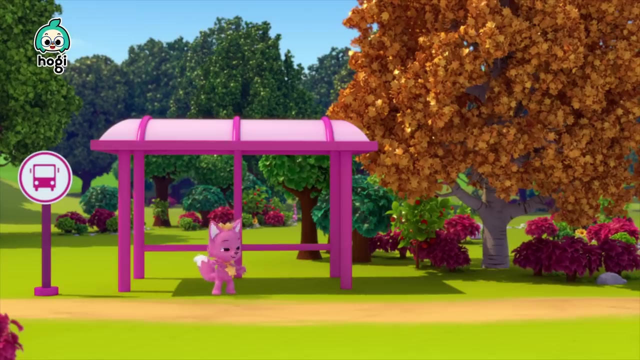 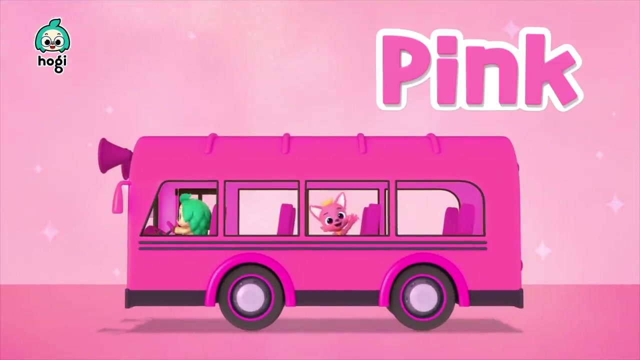 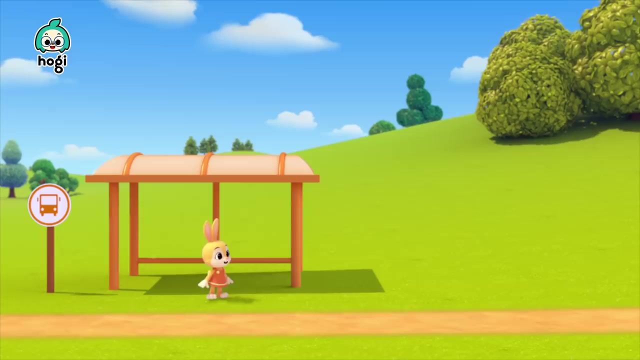 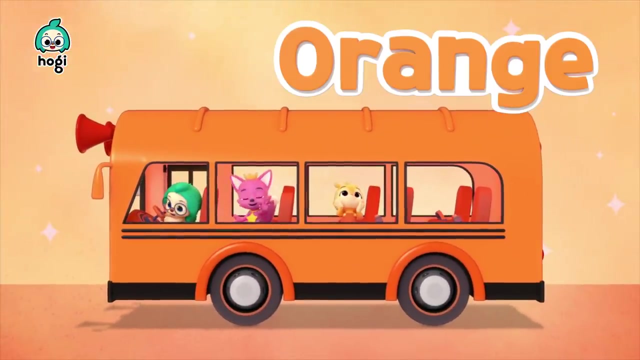 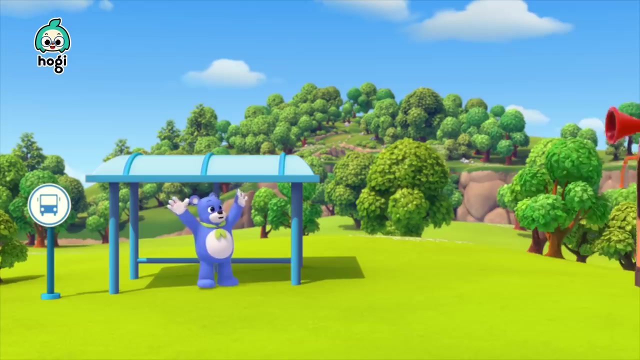 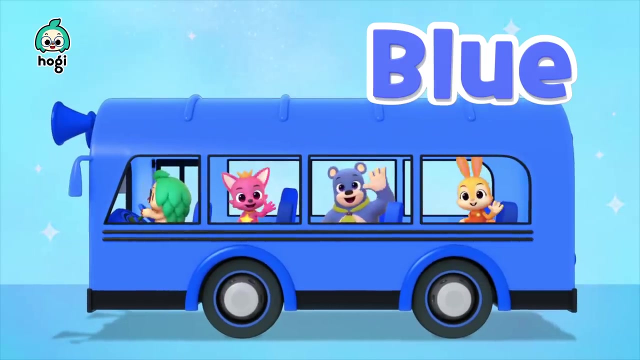 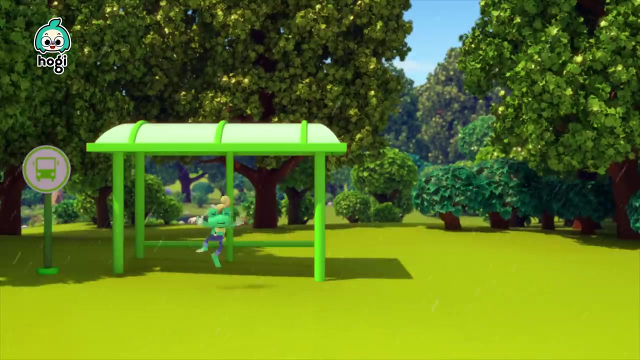 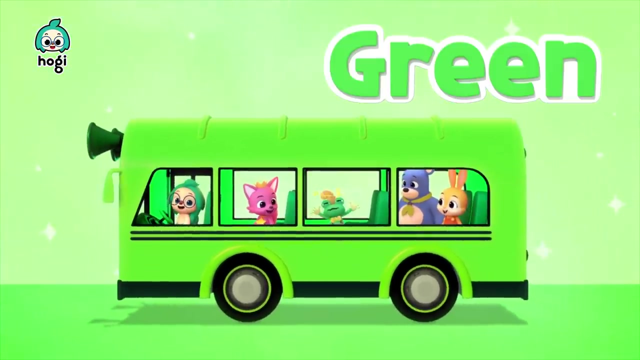 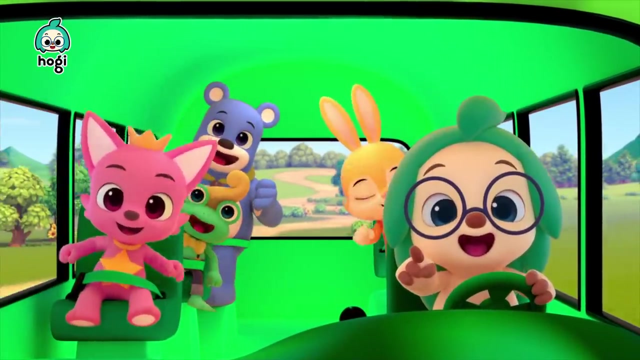 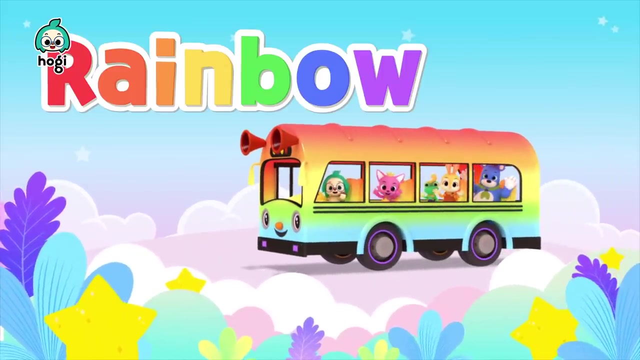 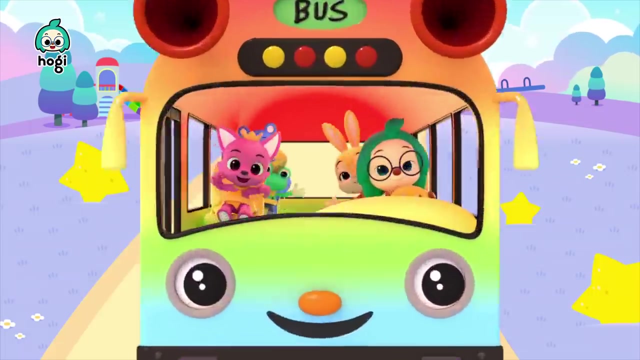 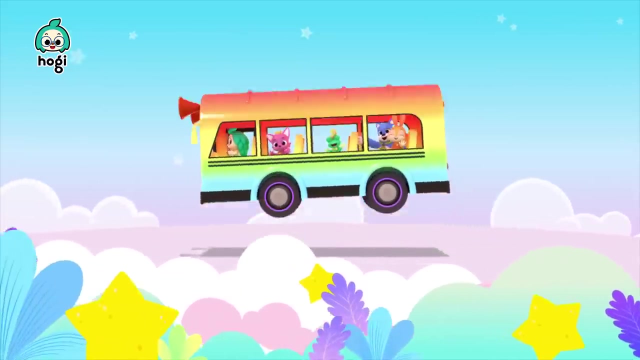 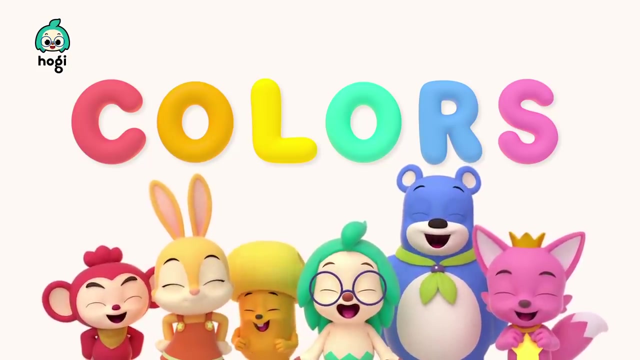 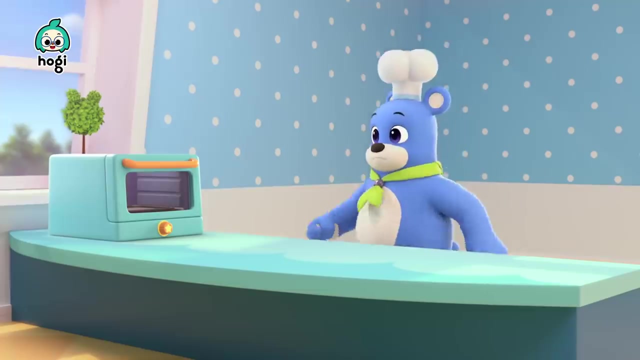 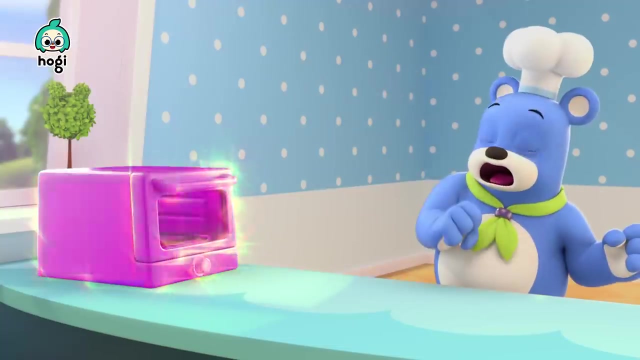 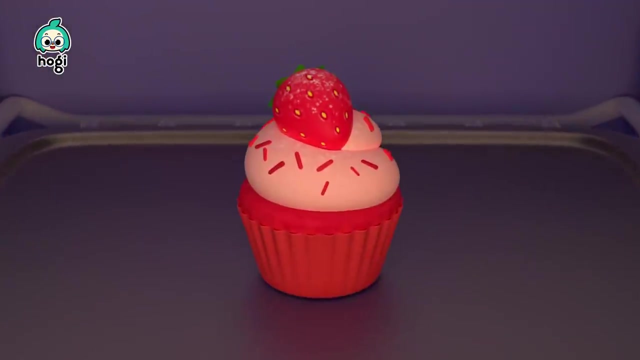 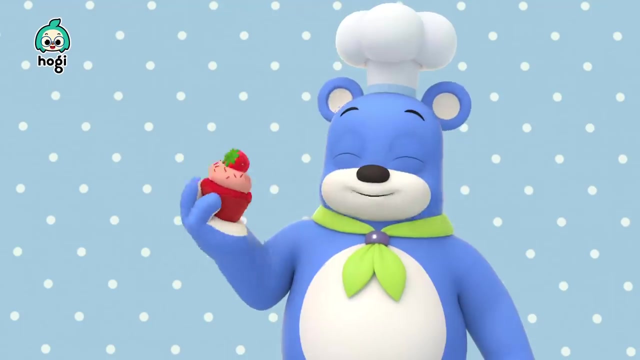 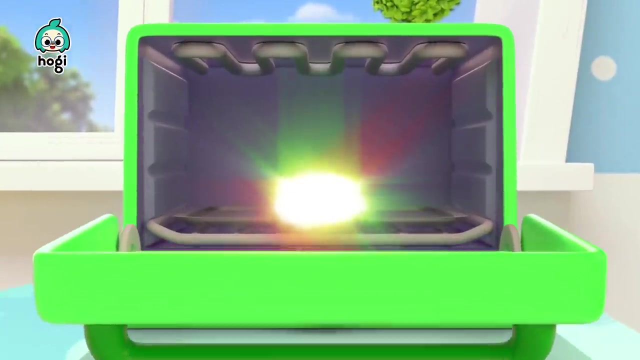 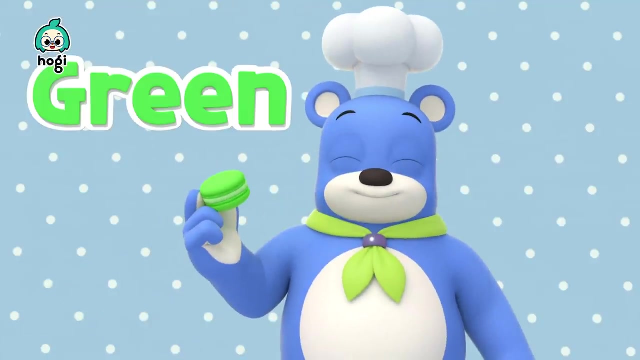 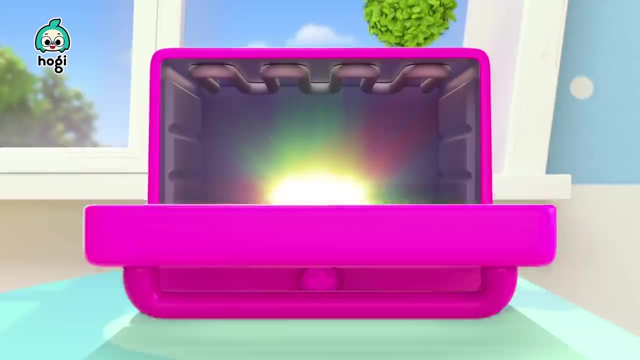 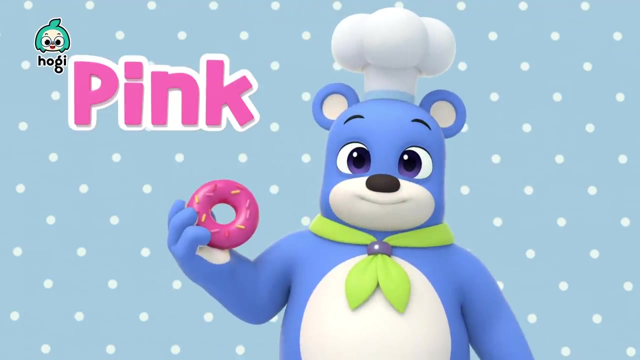 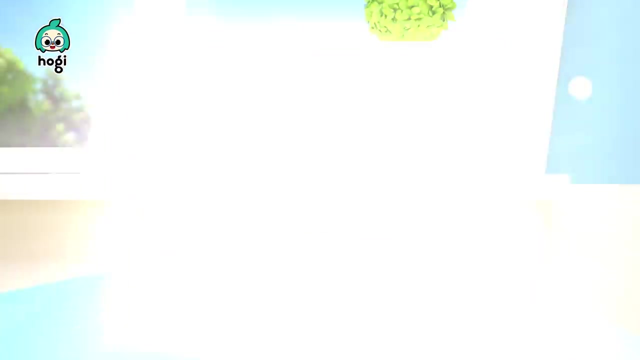 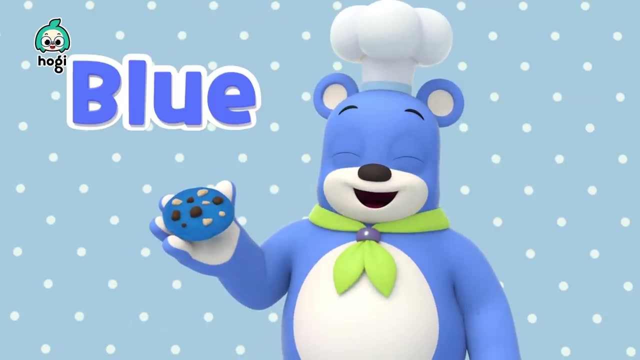 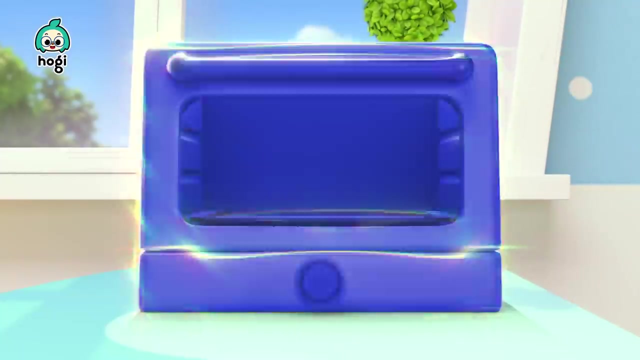 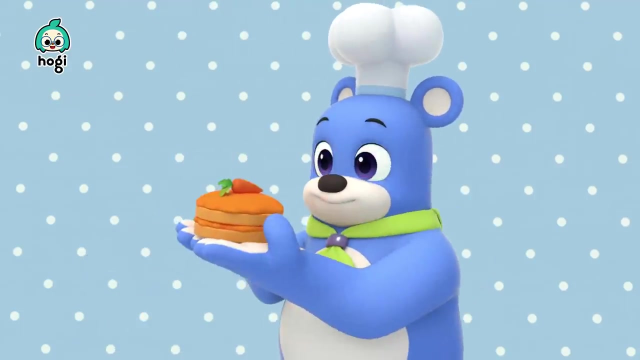 Wrong Wrong, Wrong, Wrong, Wrong, Wrong Wrong. Yellow lion Colors- Pink, Orange, Blue, Blue, Green, Rainbow. Yellow Colors- Blue, Red, Green, Blue, Pink, Blue, Orange, Orange. 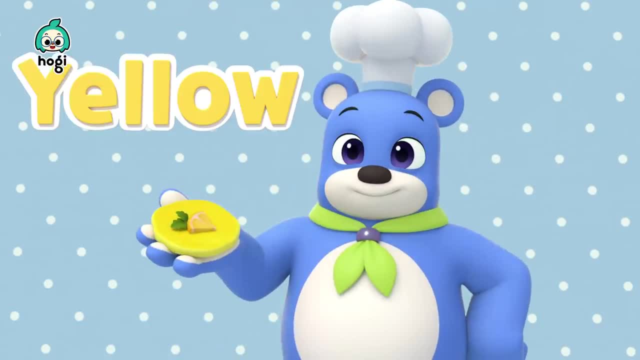 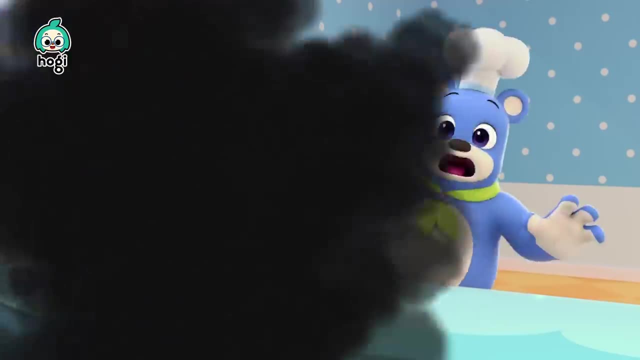 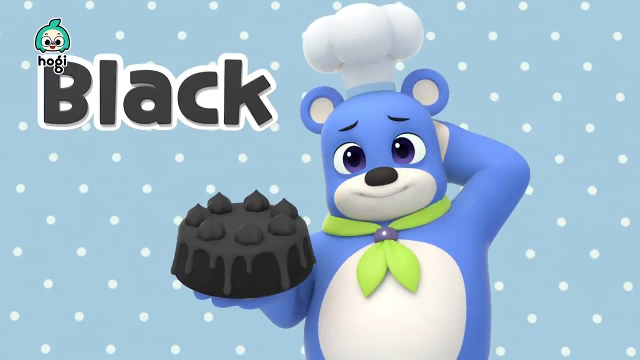 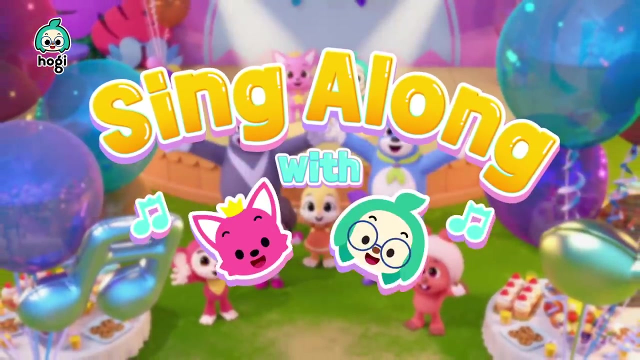 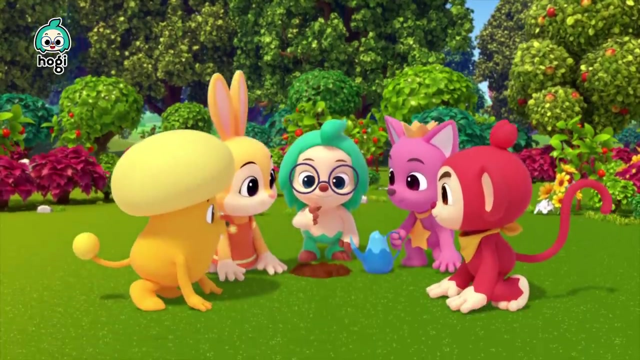 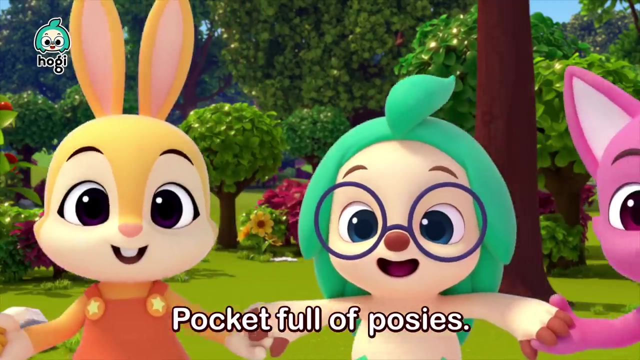 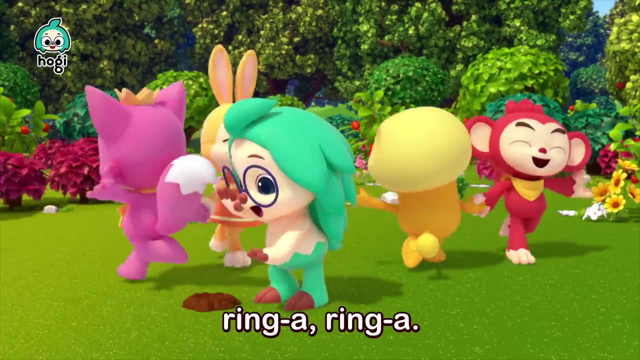 Yellow, Blue, Blue Sing along with Pinkfong and Hoagie. Ringo, Ringo Roses Pocket full of posies. Jump, Jump. We all fall down. Ringo, Ringo, Ringo, Ringo, Ring, Ring, Ring, Ringo, Ringo, Ringo, Ringo. 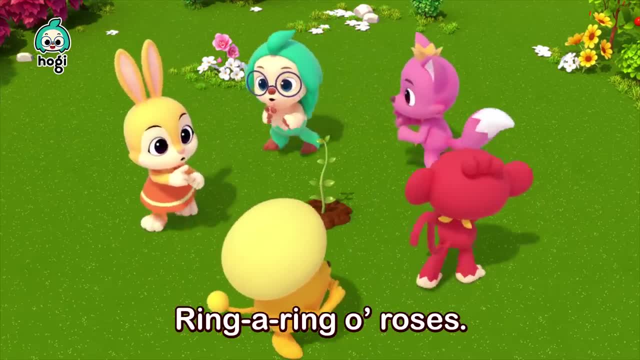 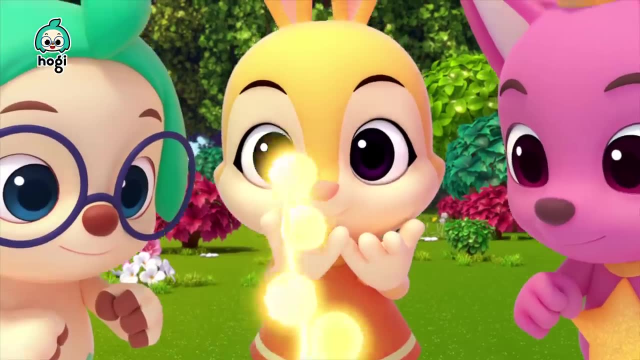 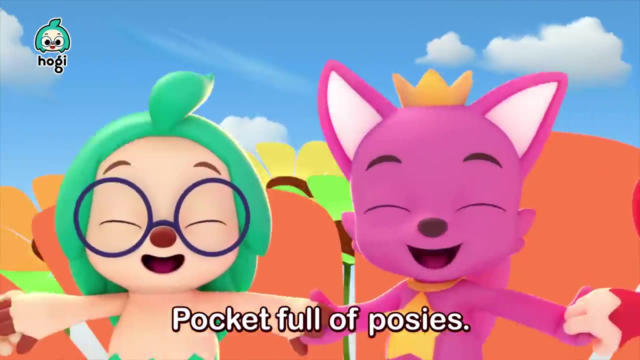 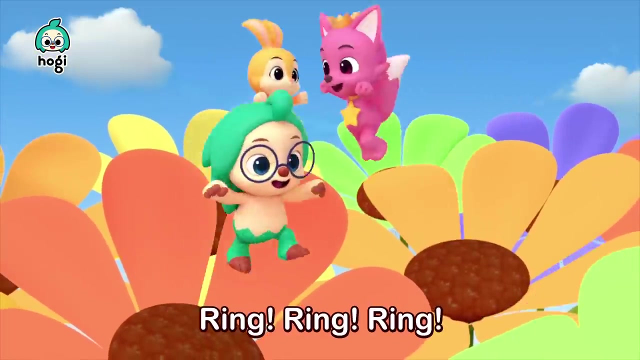 Ring, Ring, Ring, Ringo, Ringo Roses. Pocket full of posies, Jump Jump, We all fall down. Ringo, Ringo Roses. Pocket full of posies, Jump Jump, We all fall down. Ringo, Ringo, Ringo, Ringo, Ring, Ring, Ring, Ringo, Ringo, Ringo, Ringo. 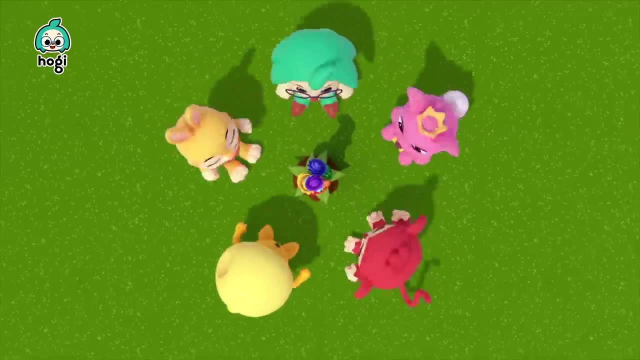 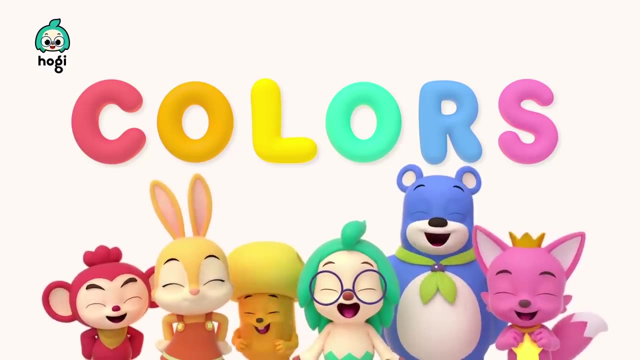 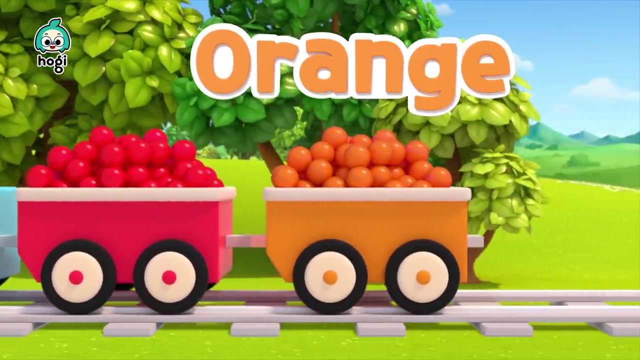 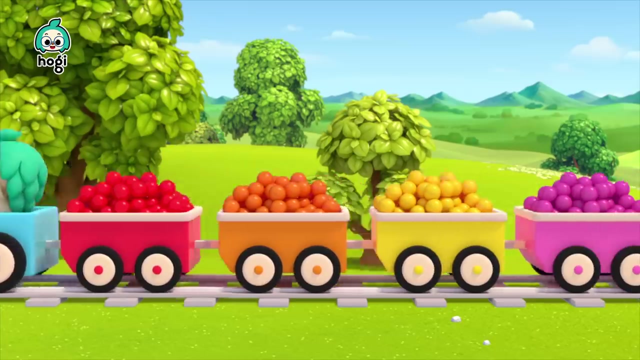 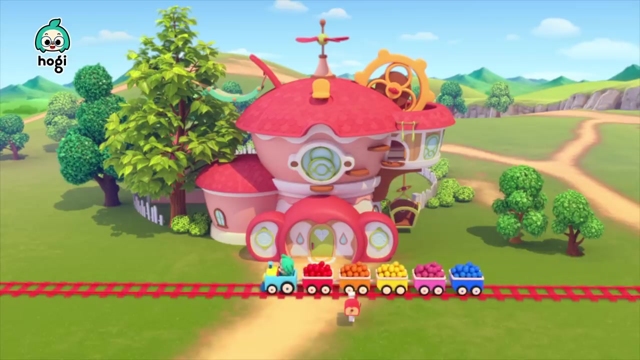 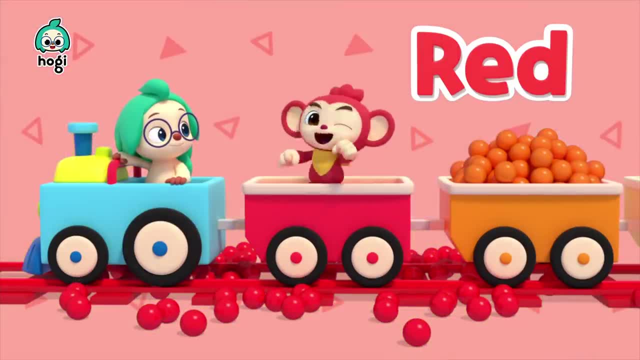 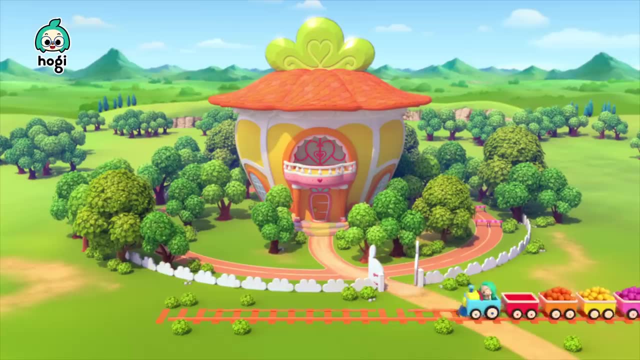 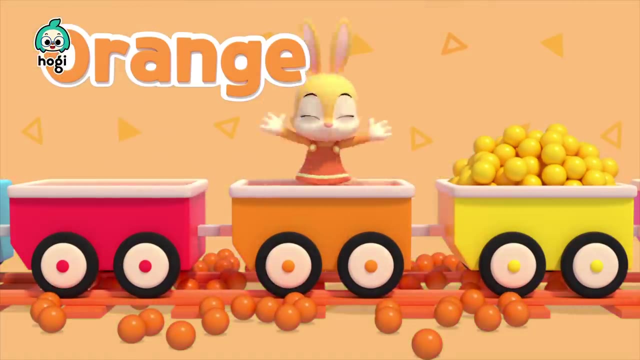 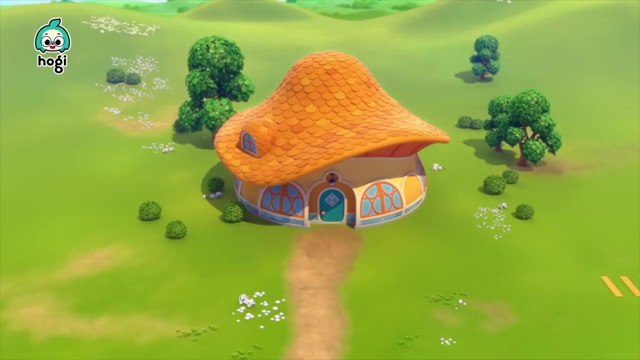 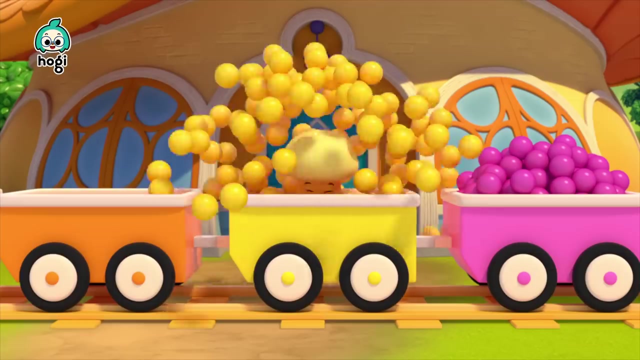 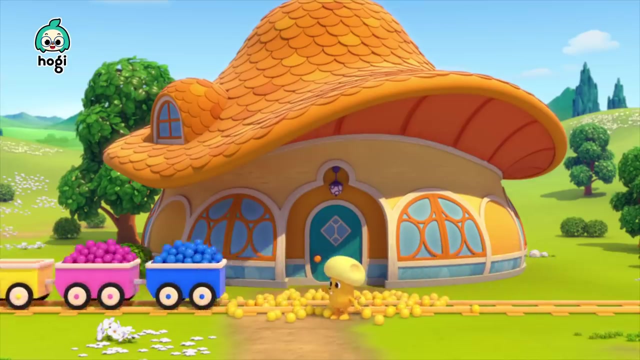 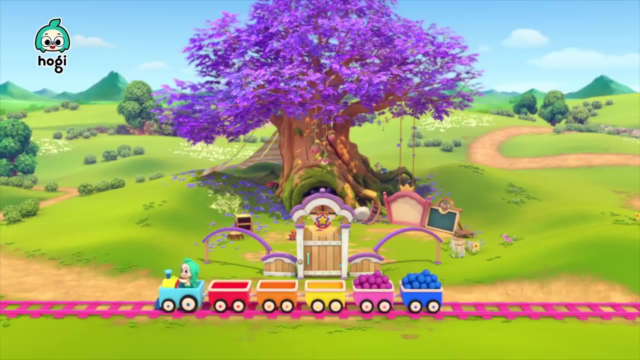 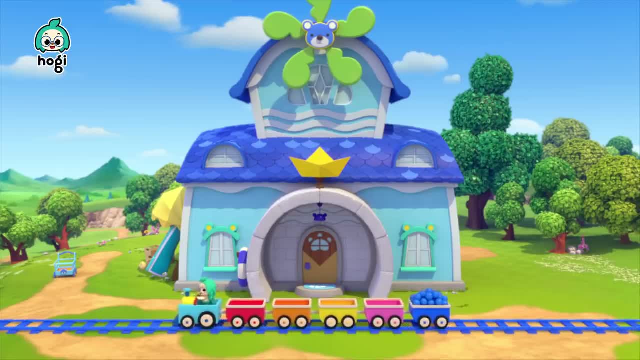 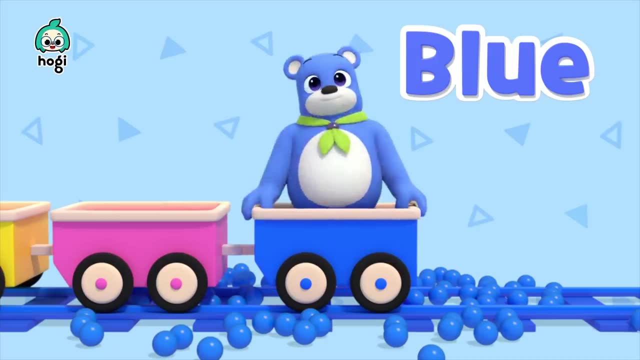 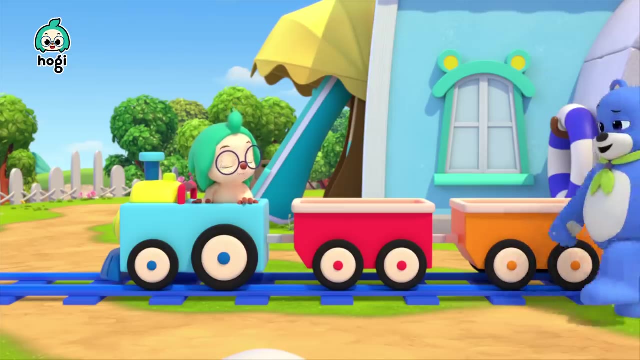 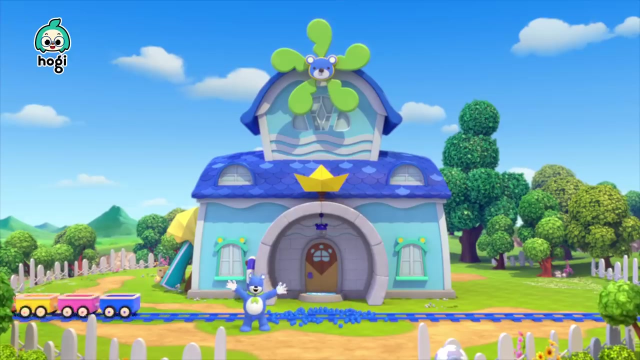 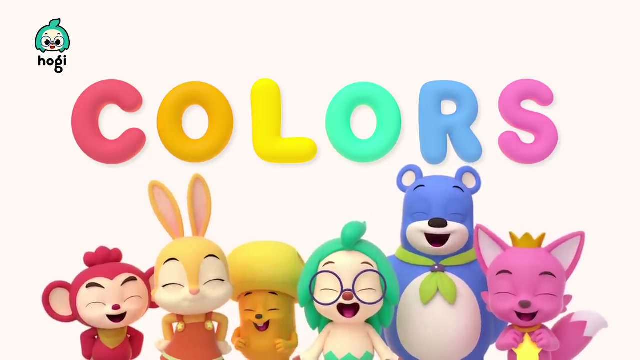 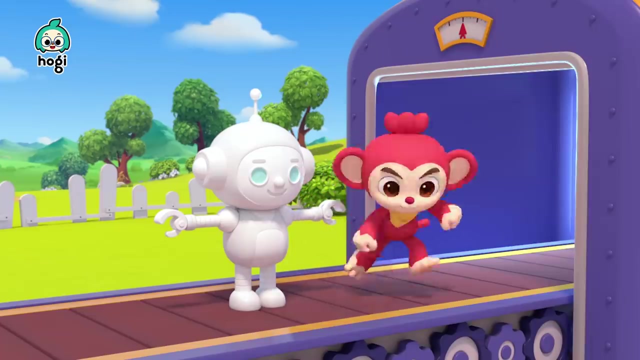 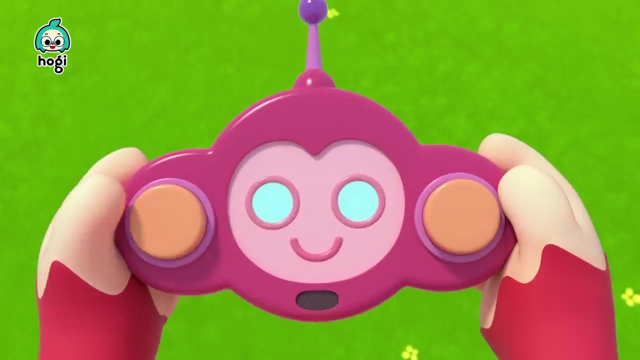 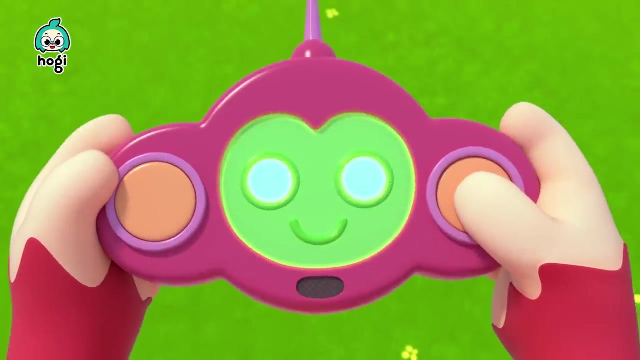 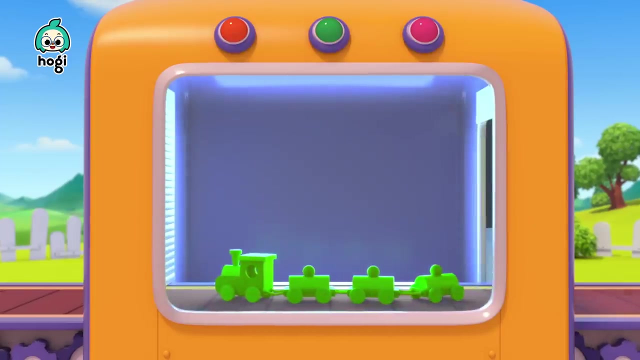 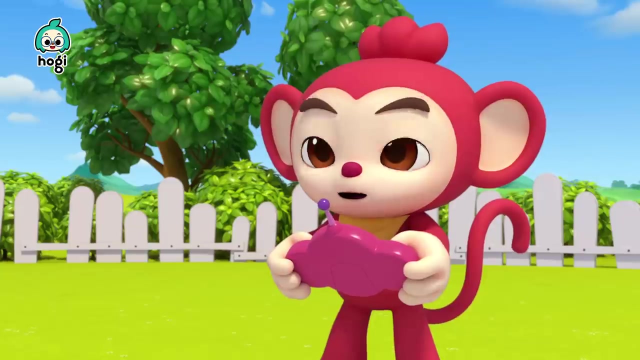 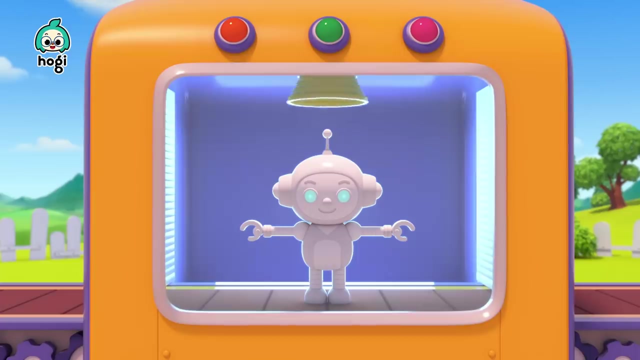 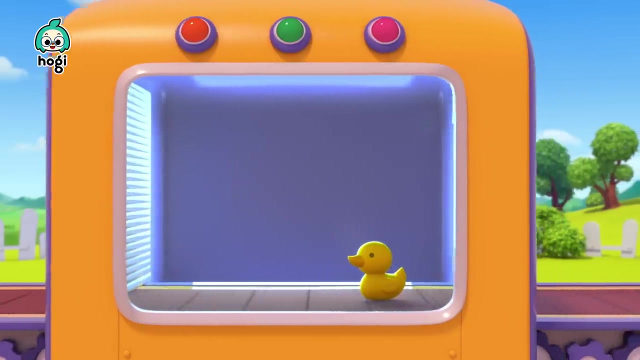 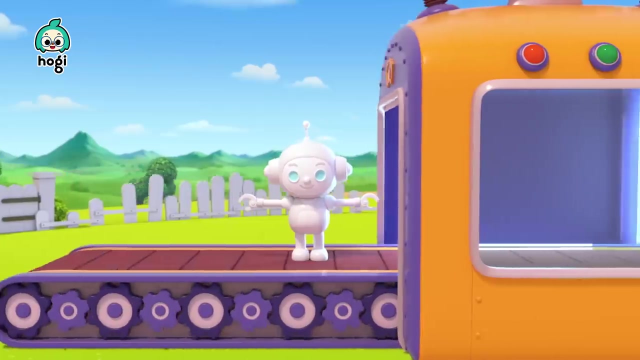 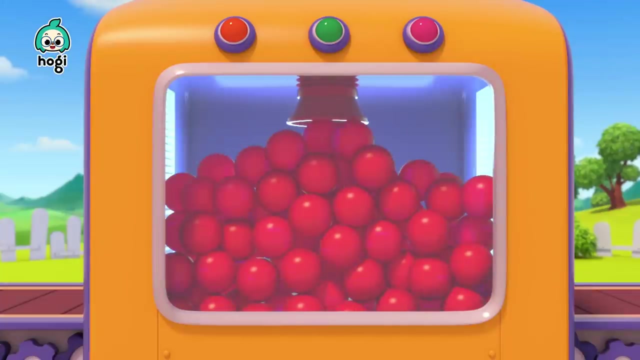 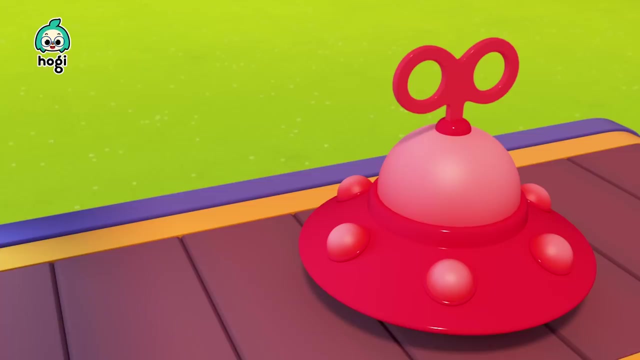 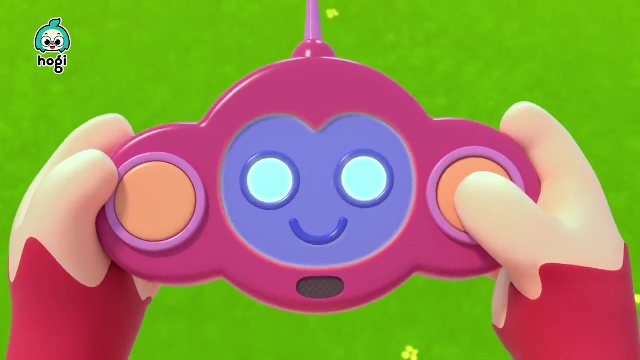 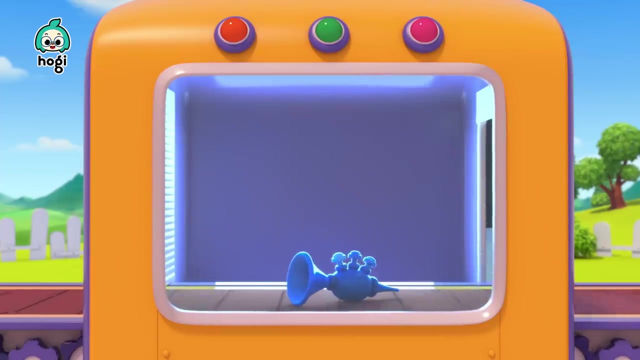 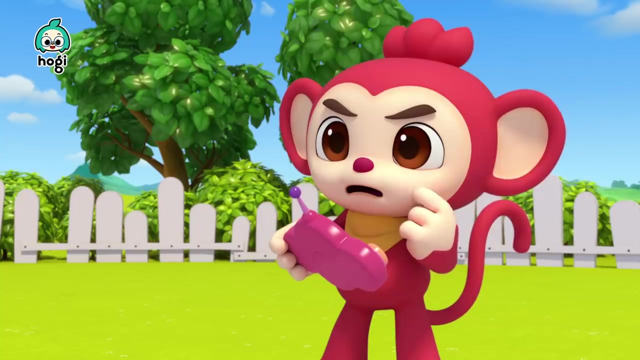 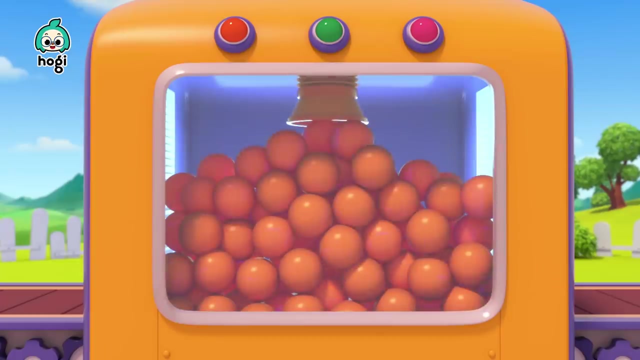 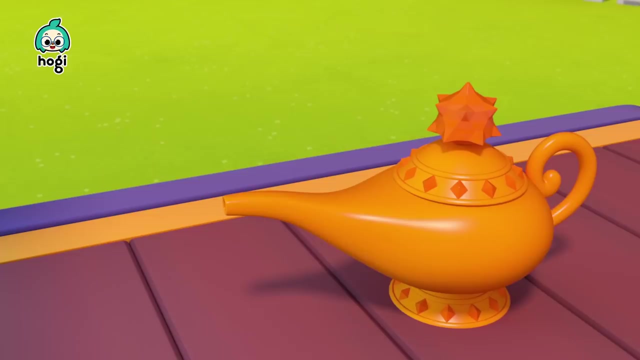 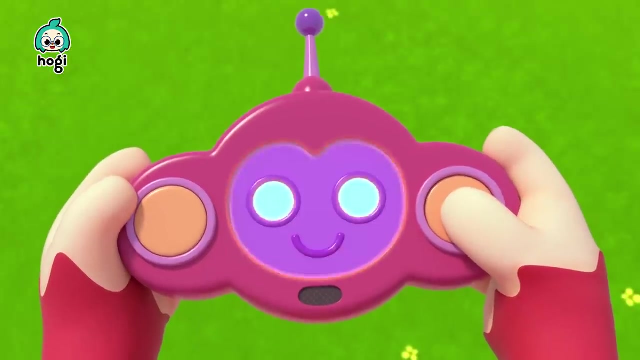 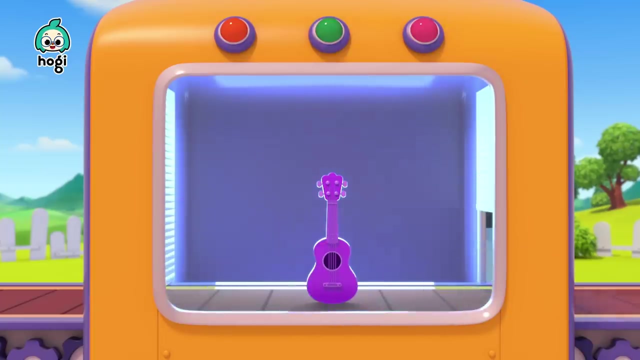 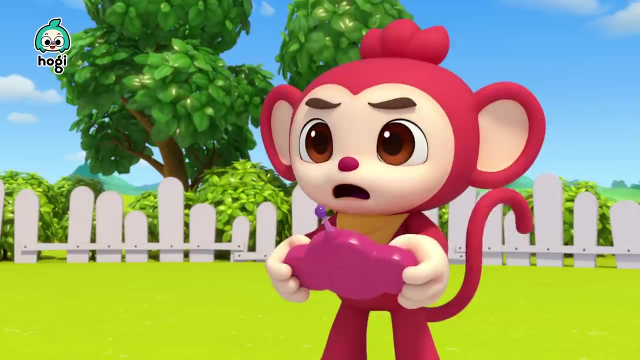 Blue, Yellow. Yeah, Colors: Green, Yellow, Green, Green, Yellow, Yellow, Red, Red, Blue, Blue, Blue, Blue, Blue Blue Blue, Orange, Blue, Blue, Blue, Blue, Purple Blue. 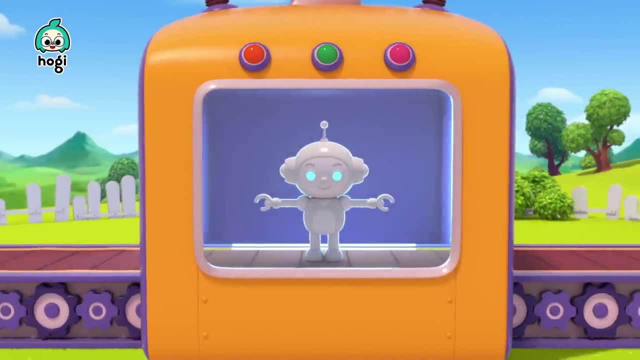 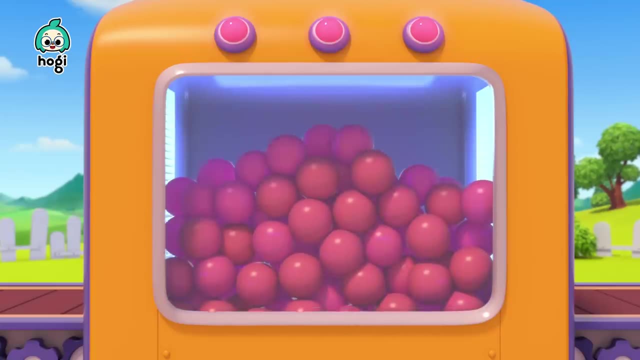 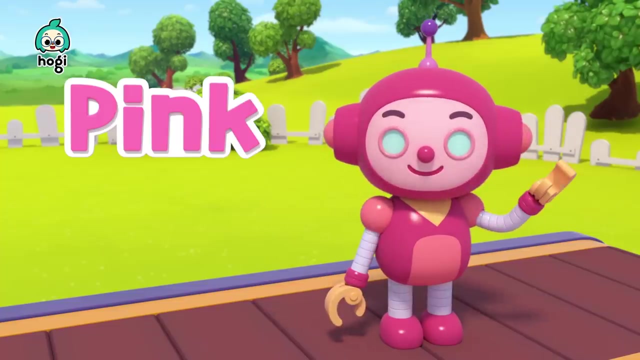 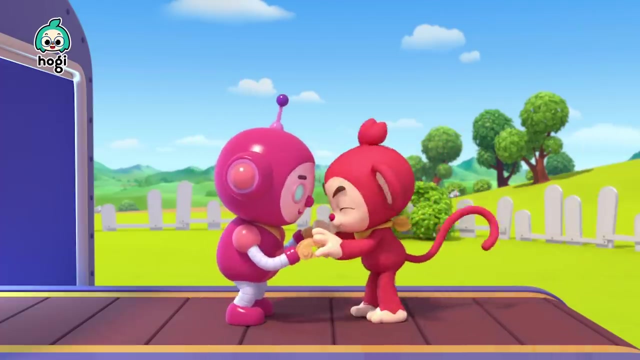 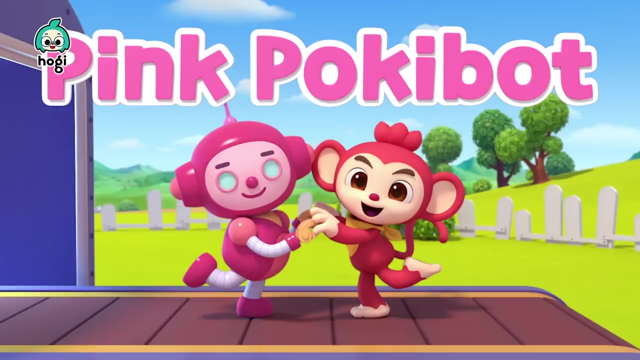 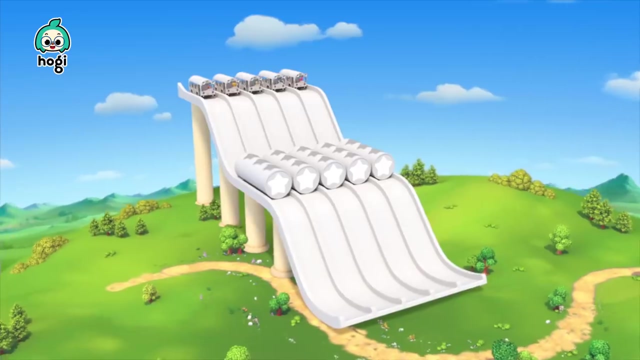 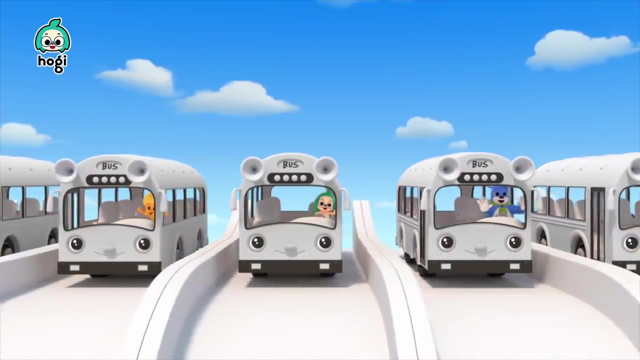 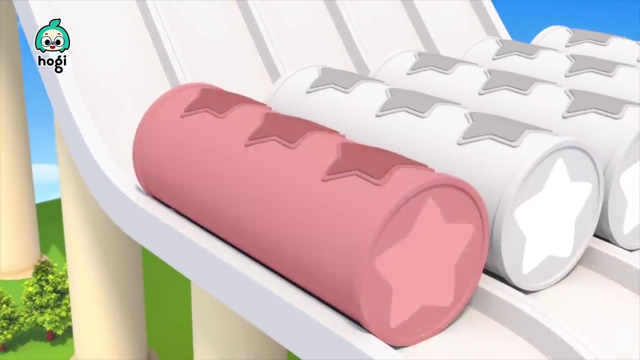 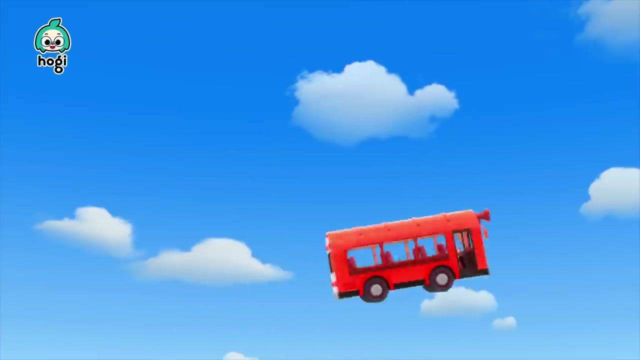 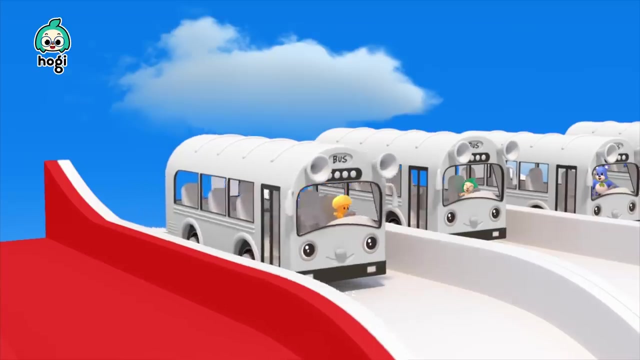 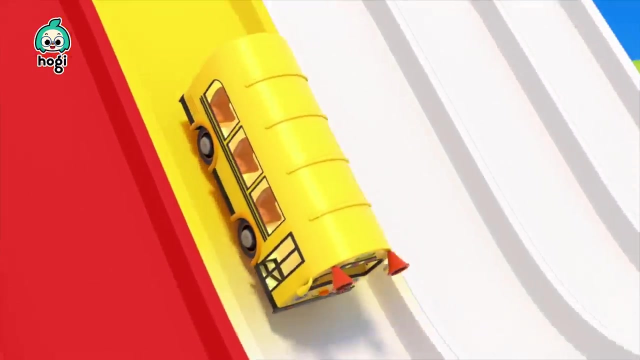 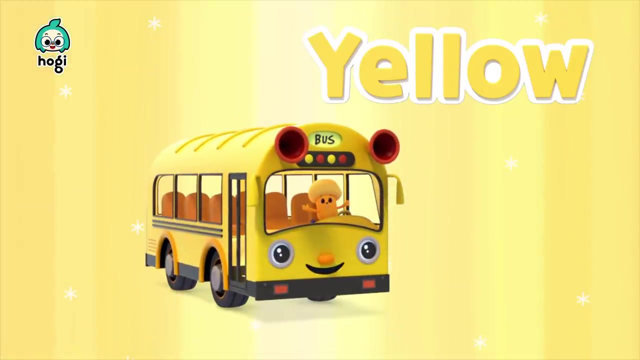 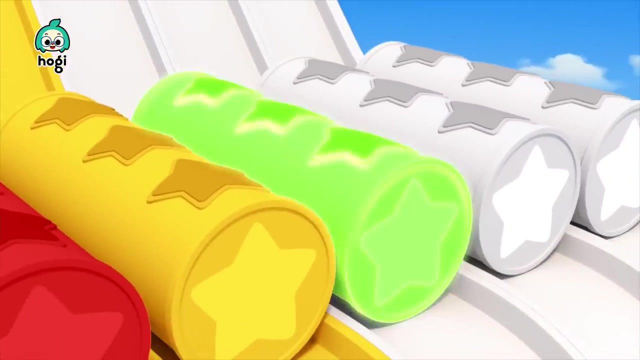 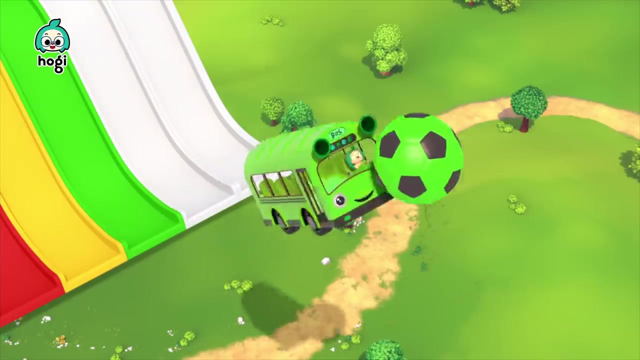 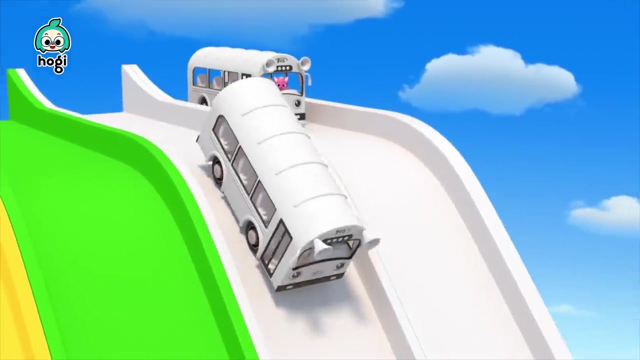 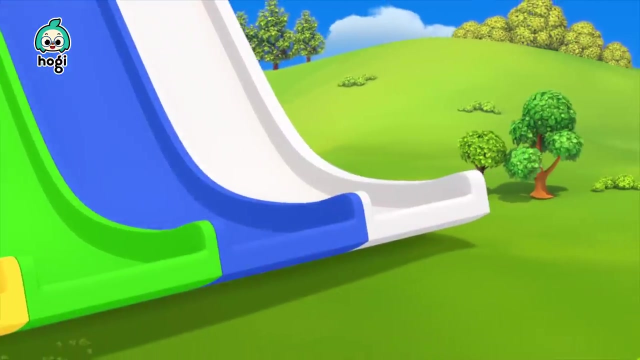 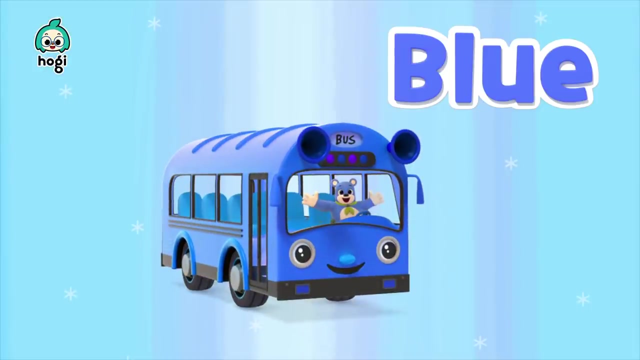 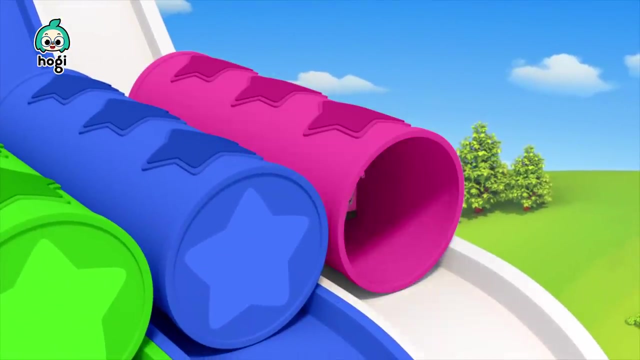 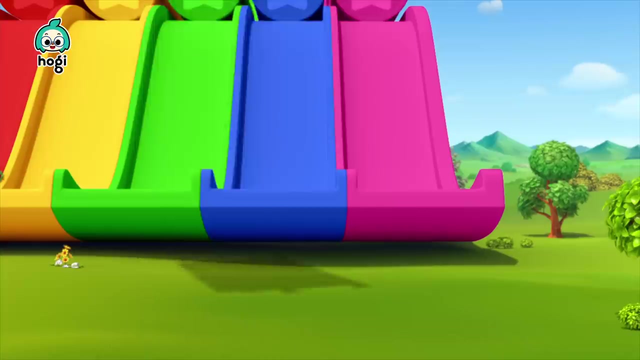 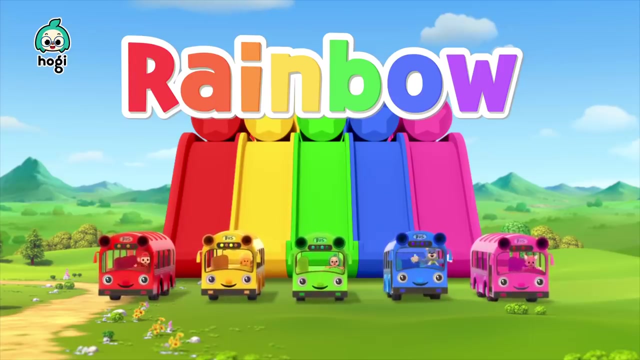 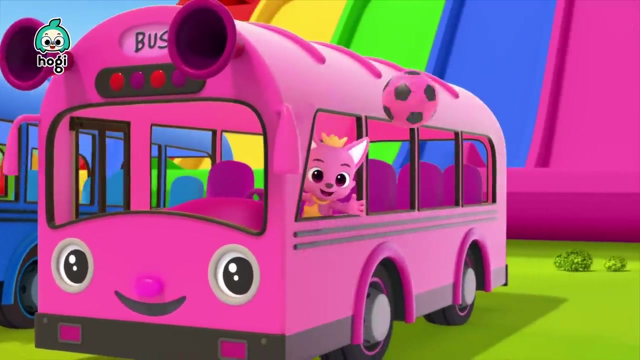 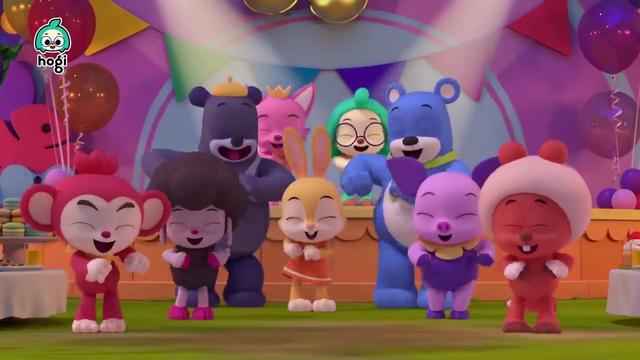 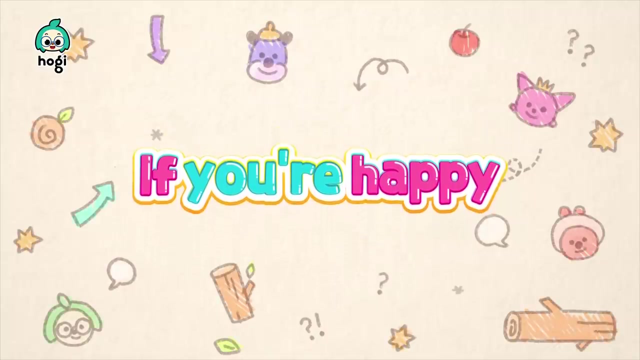 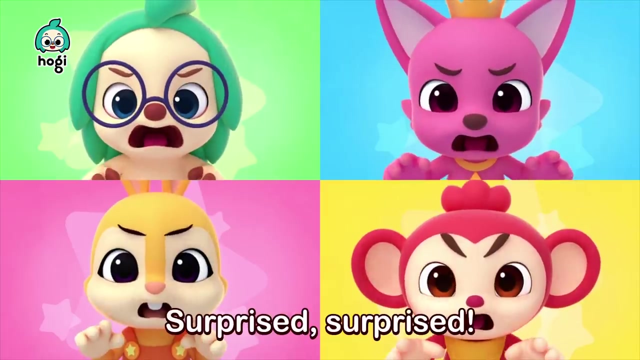 Blue, Blue, Pink, Blue, Pink, Pink, Pink, PokéBot, Pink, PokéBot Colors: Red, Yellow, Green, Blue, Blue, Pink, Rainbow. Sing along with Pinkfong and Hoagie: Happy, Happy, Sad, Sad, Angry, Angry, Surprise, Surprise. If you're happy, happy, happy. 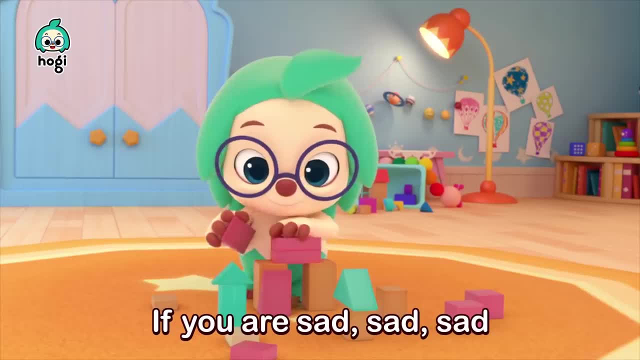 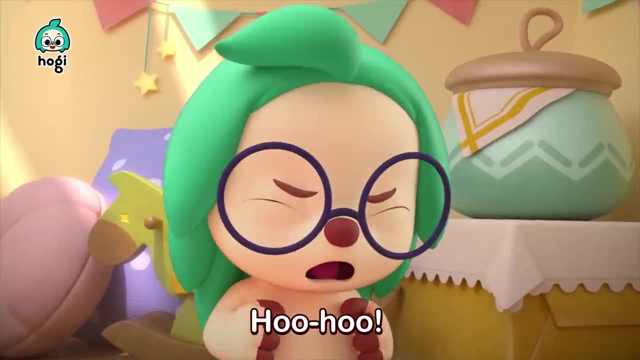 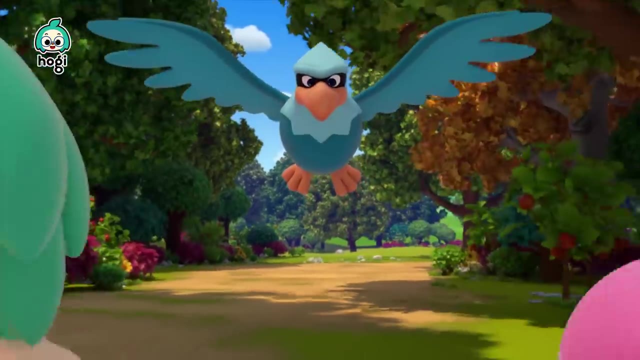 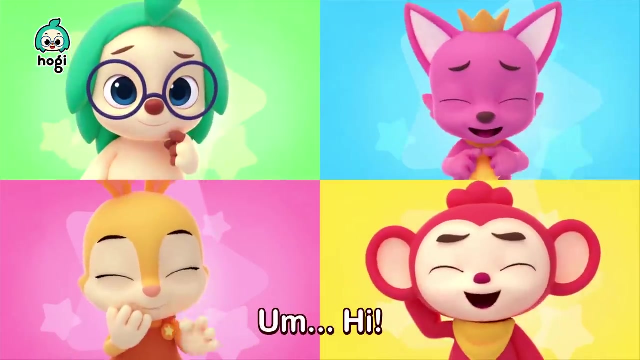 laugh out loud. If you're sad, sad, sad, cry out loud. If you're angry, angry, breathe deep. If you're surprise, surprise, jump up. Hoagie, Ha, ha, ha, ha, ha ha, Hungry, hungry, Humble, Scared, scared, Shy, shy, Sleepy, sleepy. If you're hungry, hungry. 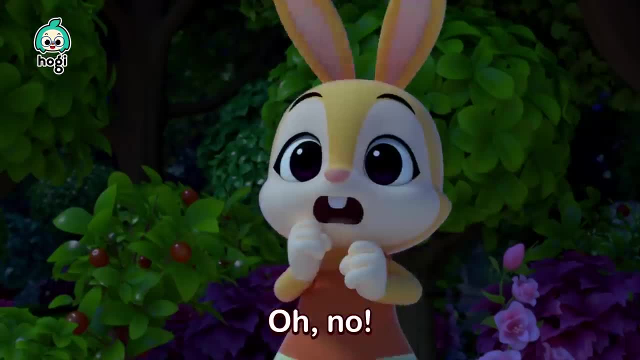 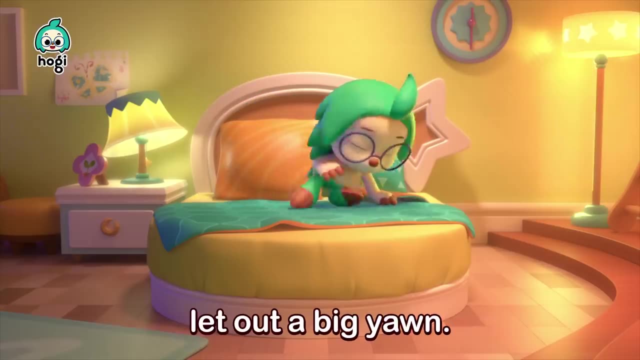 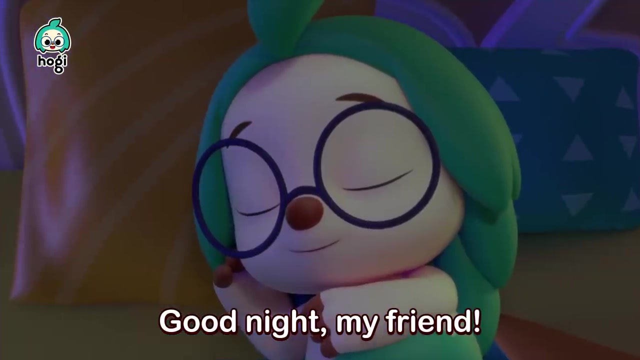 listen to your stomach rumble. If you're scared, scared, cover up your eyes. If you're shy, shy, shy, say hello. If you're sleepy, sleepy, let out a big yawn. Good night, my friends. Good night, my friends. Good night, my friends Colors. Ha ha, ha, ha, ha ha. 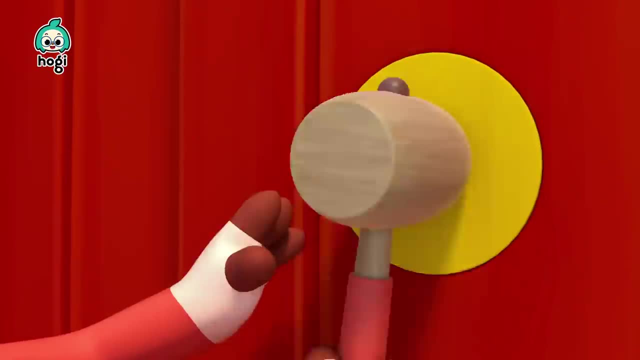 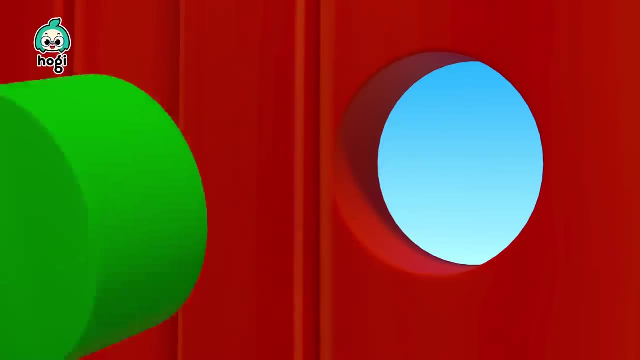 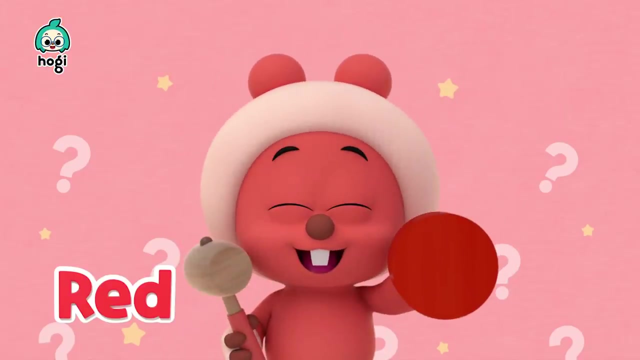 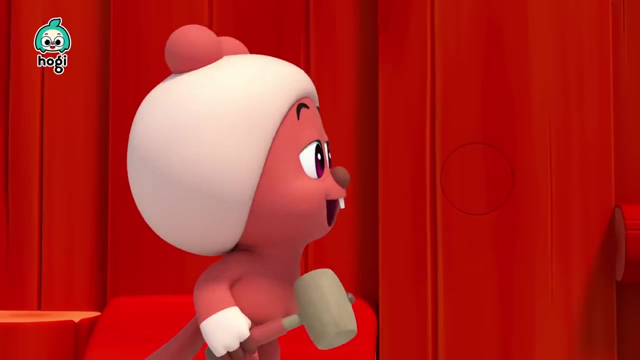 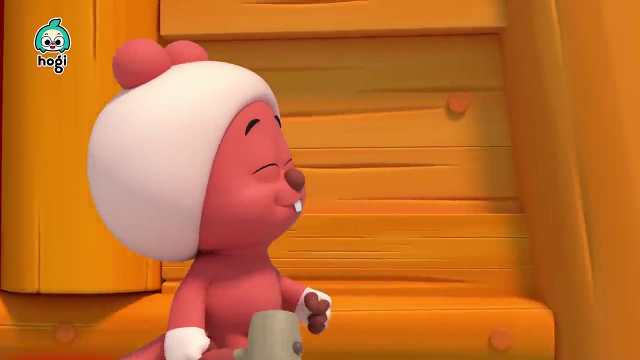 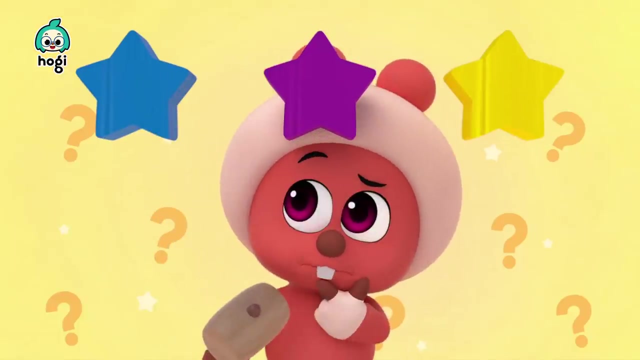 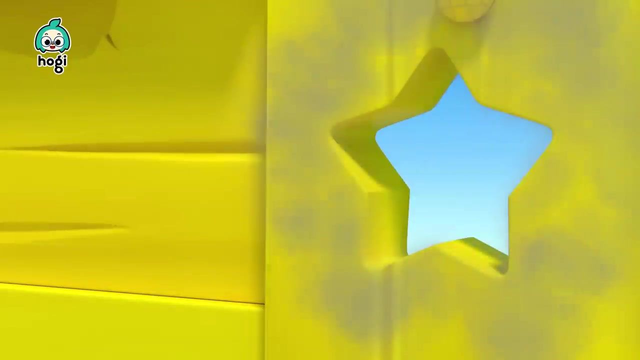 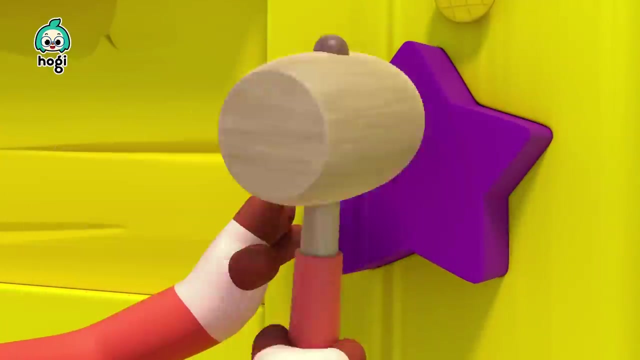 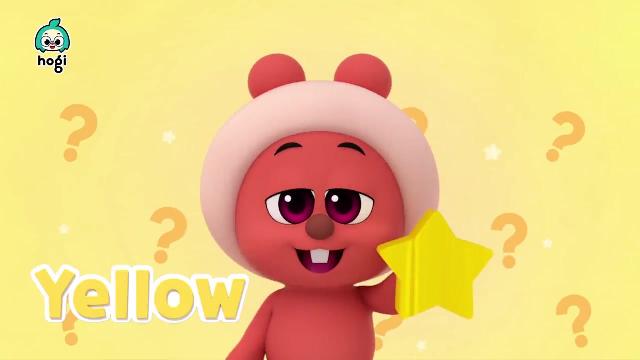 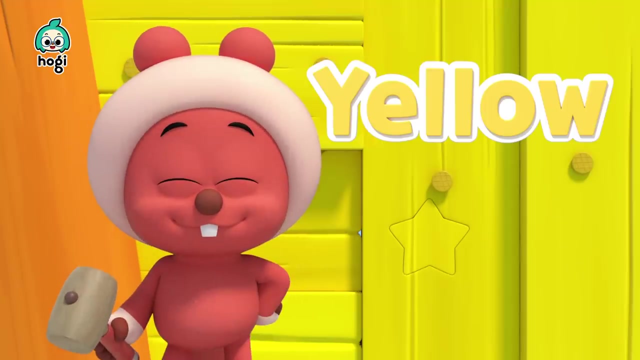 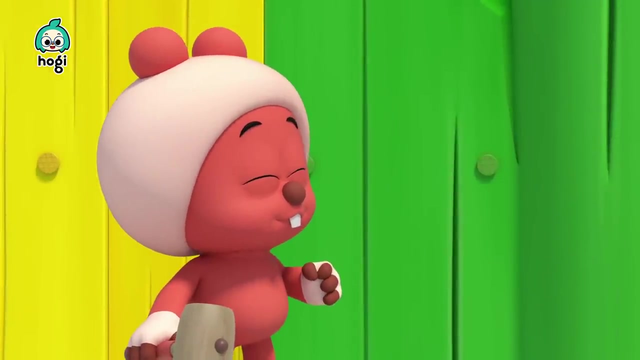 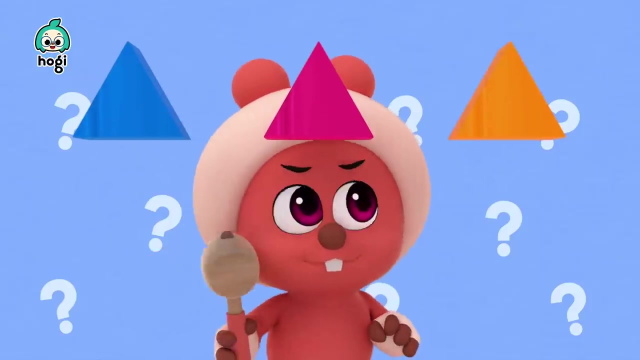 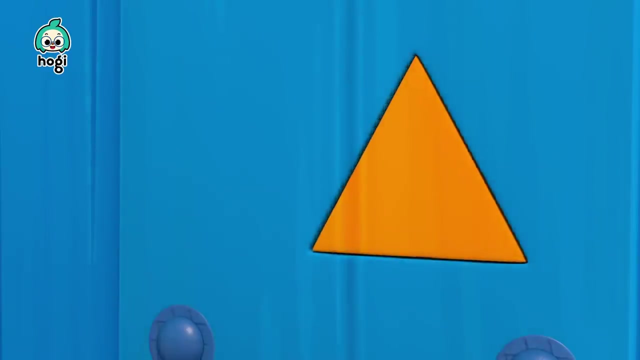 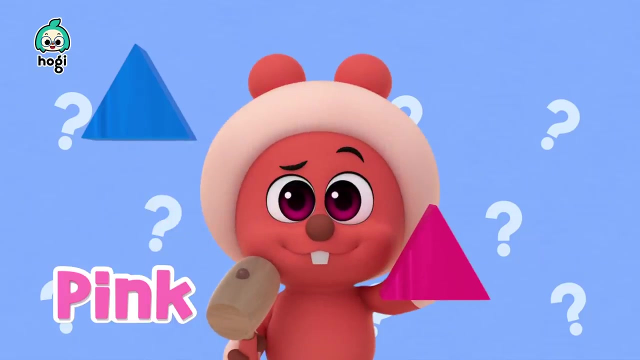 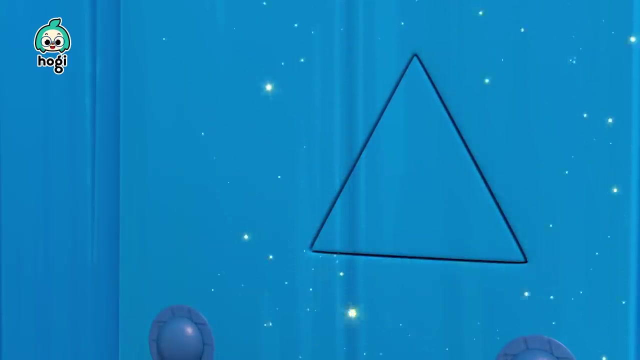 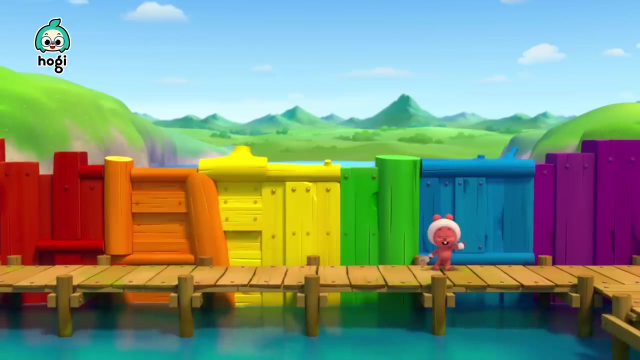 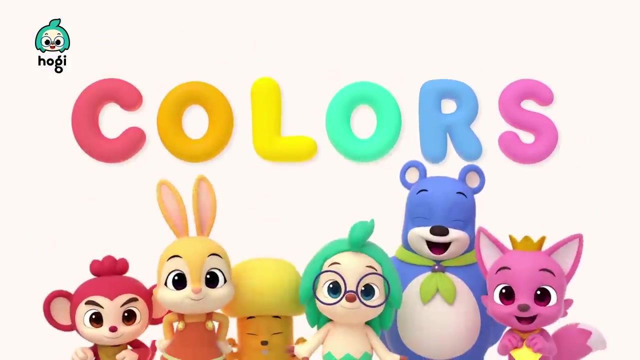 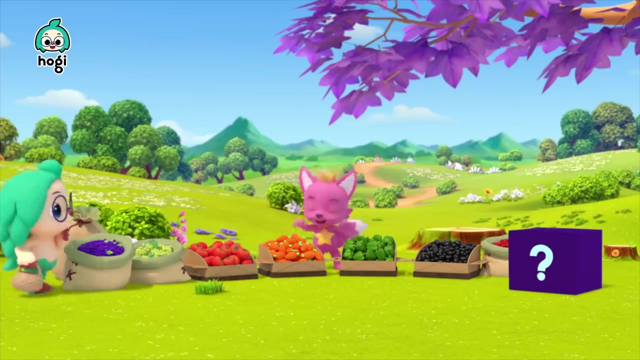 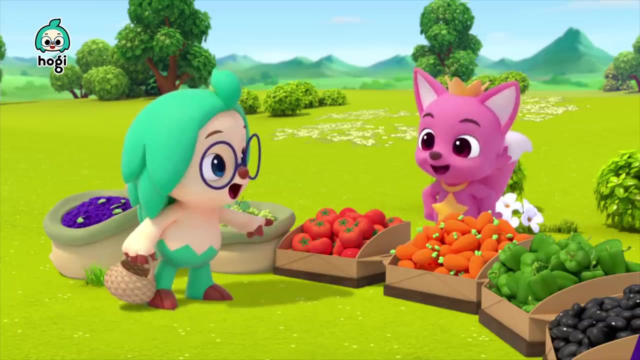 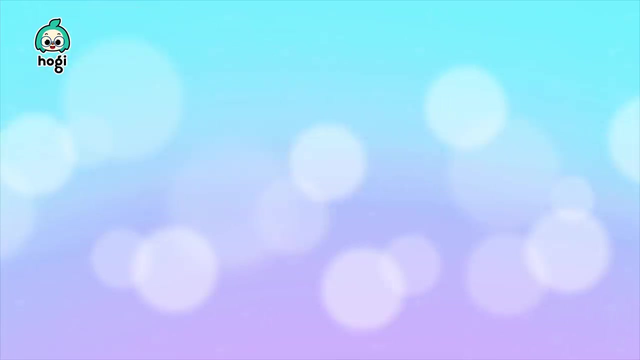 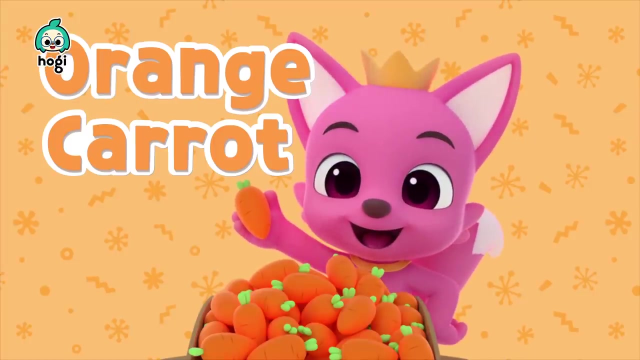 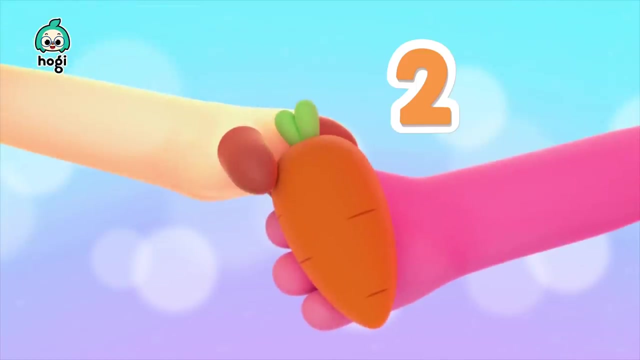 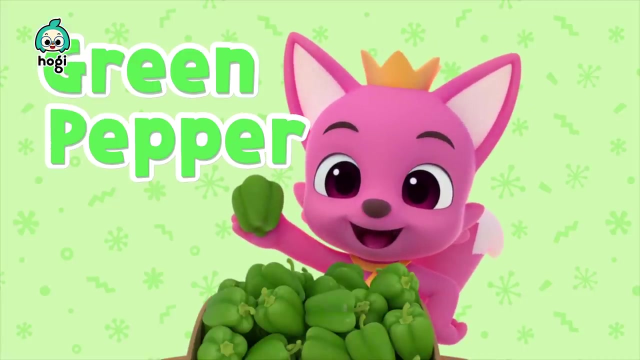 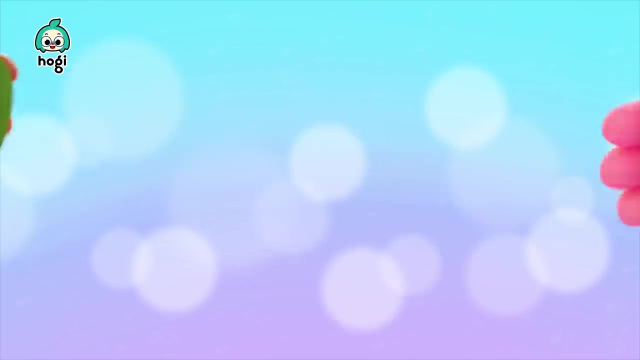 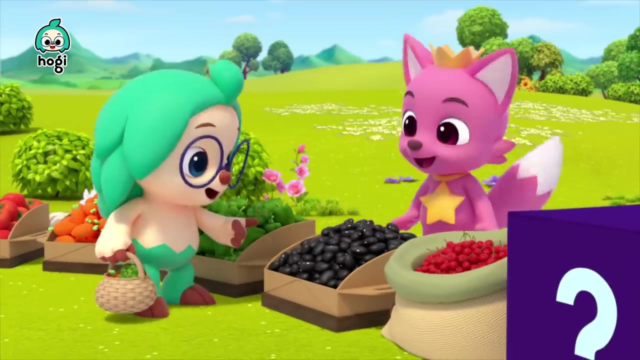 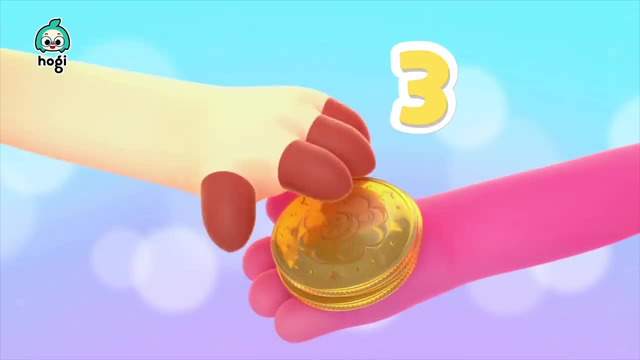 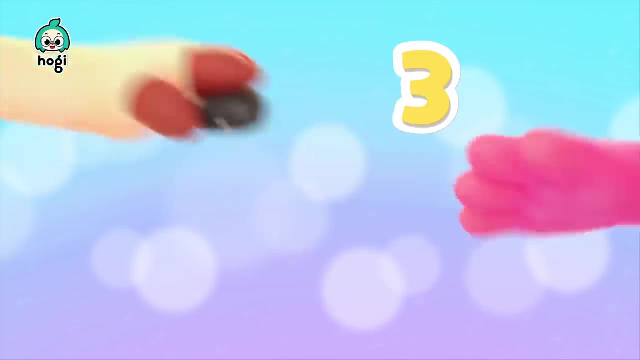 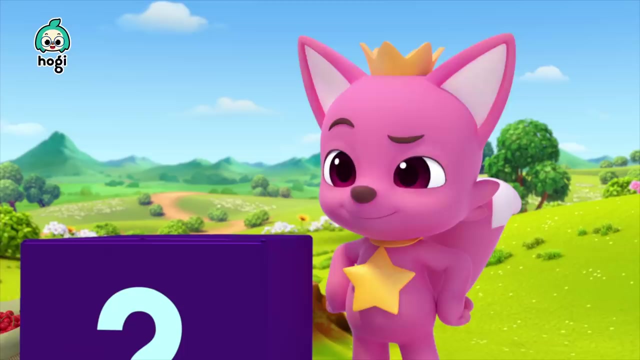 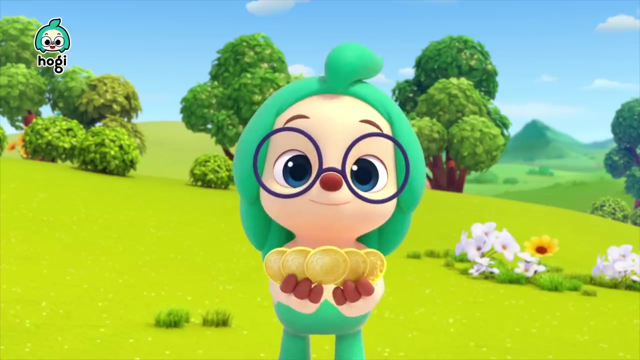 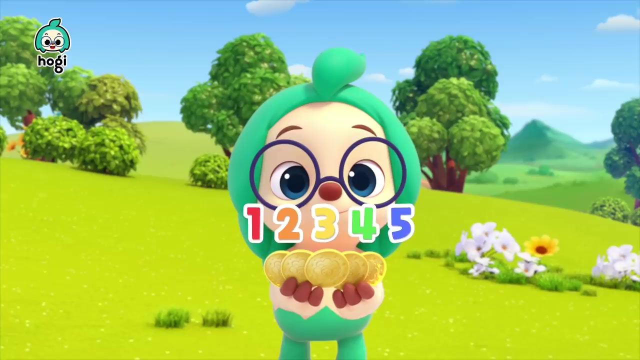 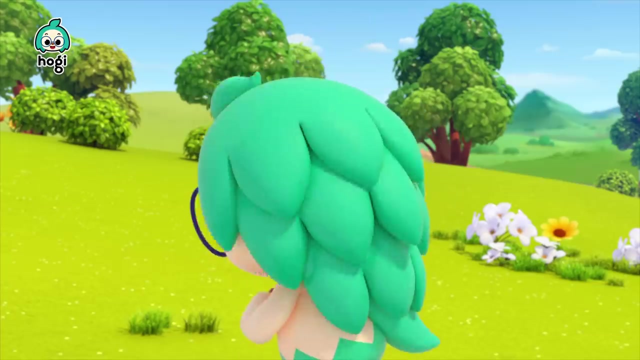 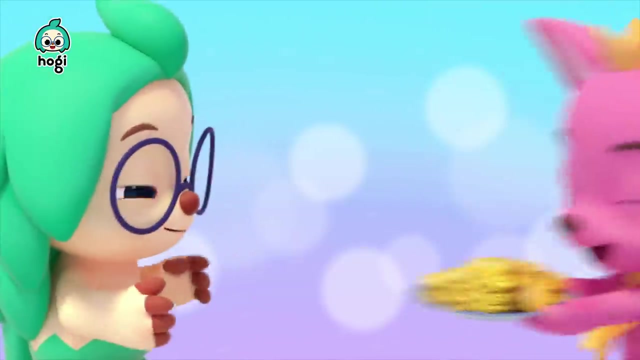 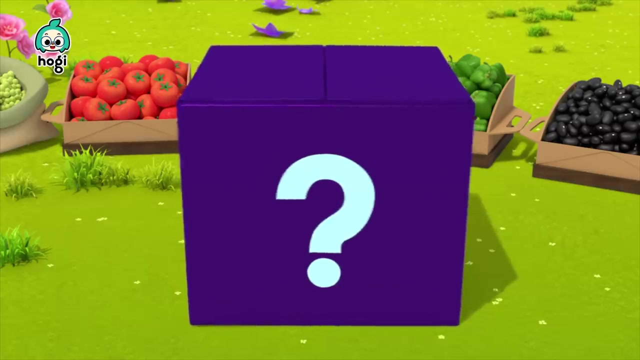 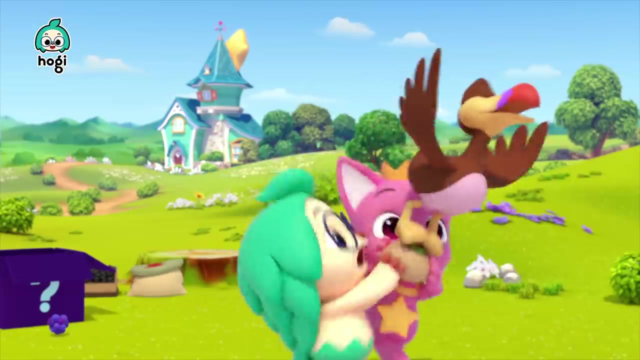 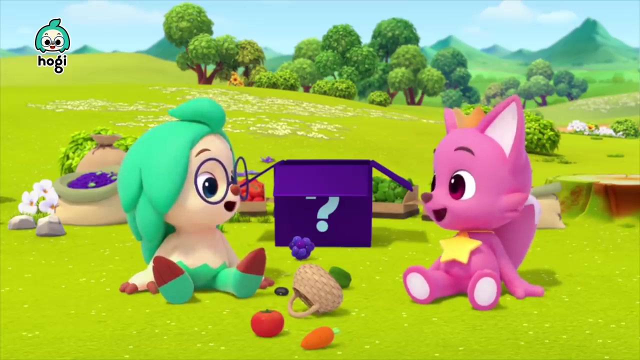 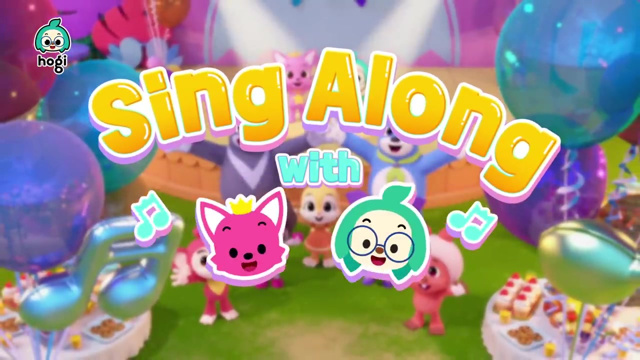 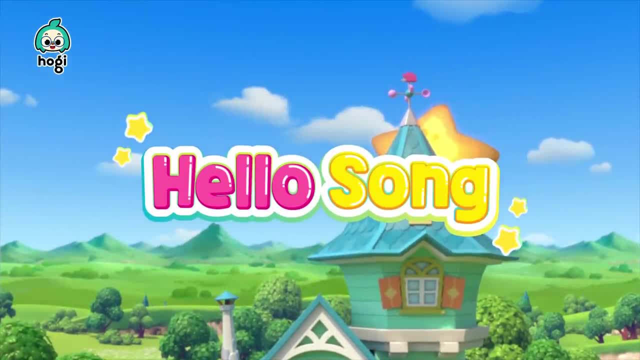 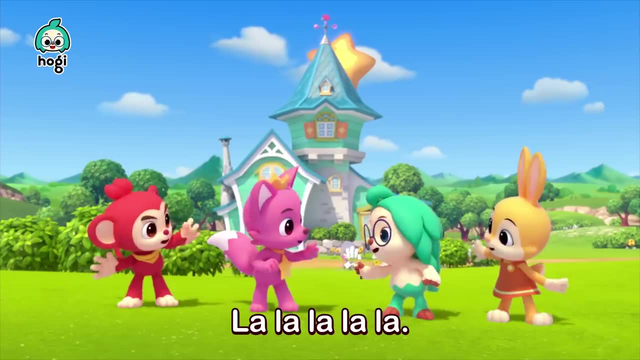 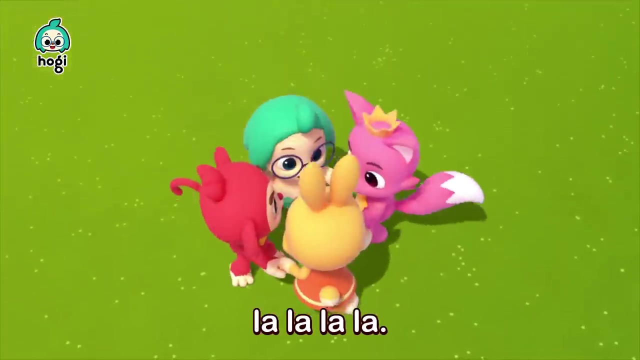 Hello with Hoagie, Right hand, la-la-la, Left hand, la-la-la. Hello. hello, Hoagie's friends, La-la-la-la-la, Let's say hello with a big, big smile. La-la-la-la-la-la-la-la, Hello, good morning. 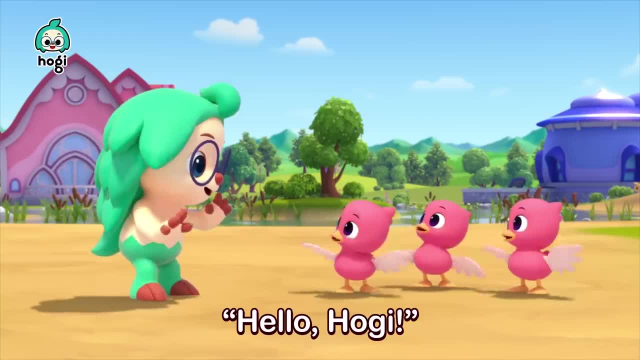 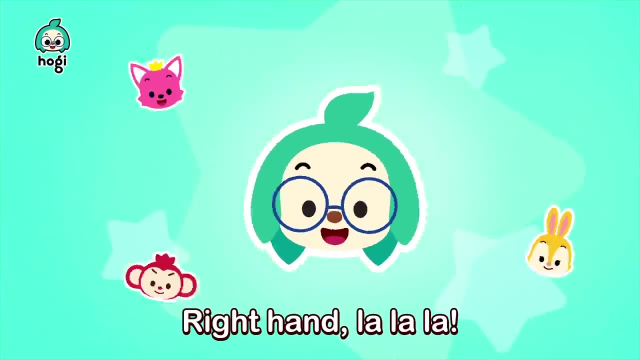 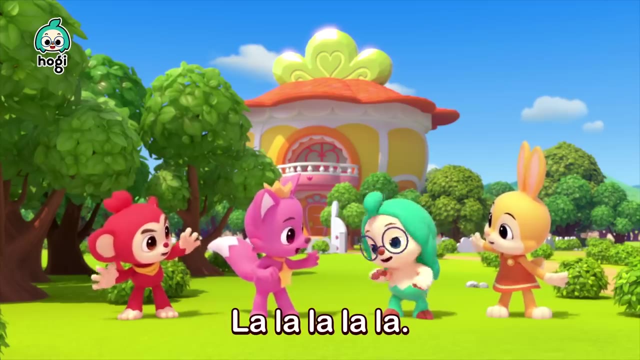 Hello Quackies, Hello Hoagie, Good morning little birds. Hey, how are you? Right hand la-la-la, Left hand, la-la-la, Hello. hello Hoagie's friends, La-la-la-la-la, Let's say hello with a big, big smile. 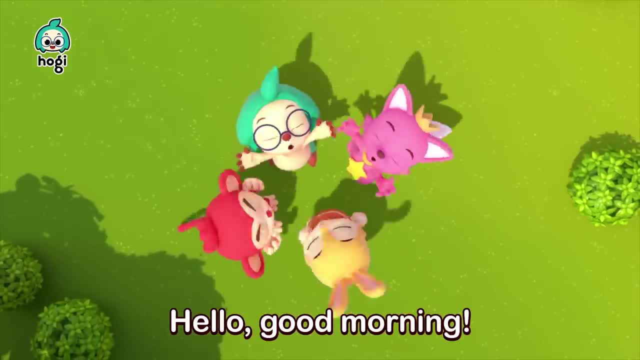 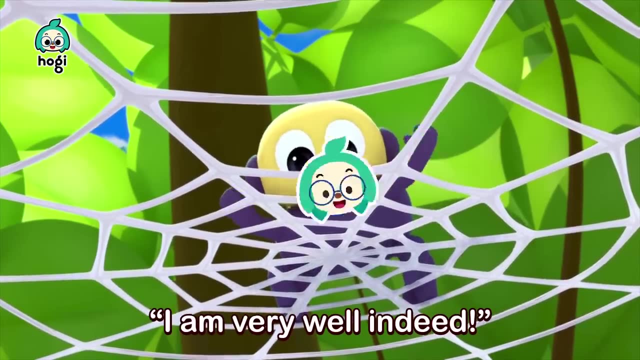 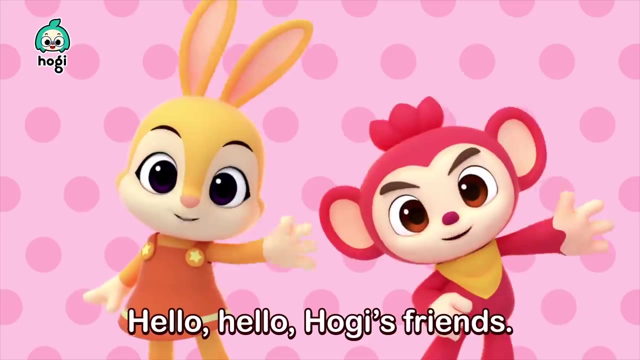 La-la-la-la-la-la-la-la. Hello, good morning, Hello, Spider. How are you? I am very well indeed. Right hand la-la-la. Left hand, la-la-la. Hello, hello, Hoagie's friends. La-la-la-la-la-la. 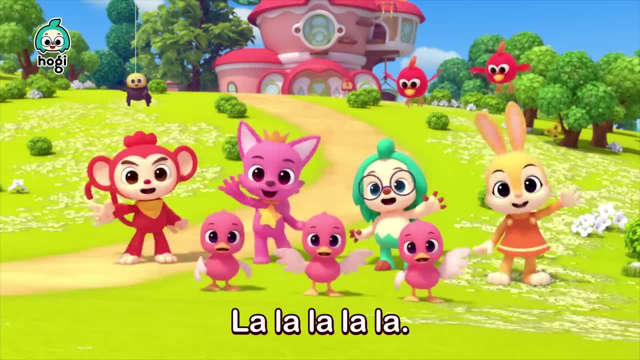 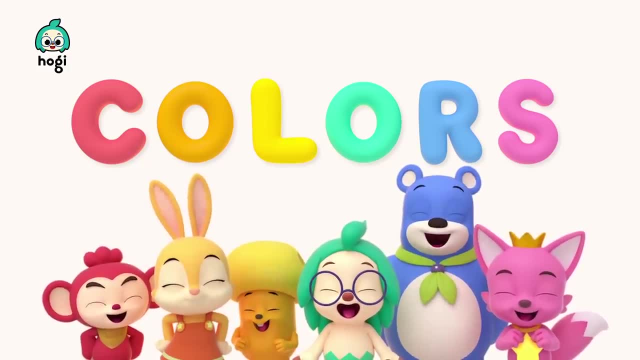 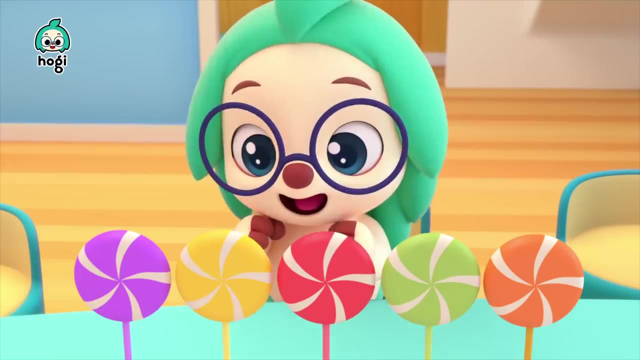 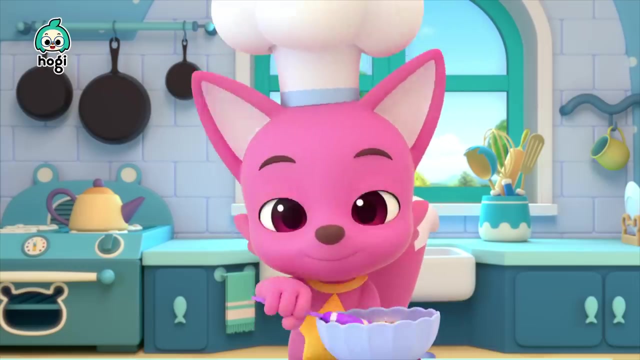 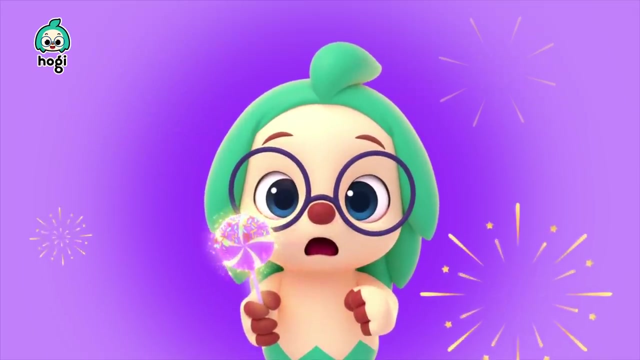 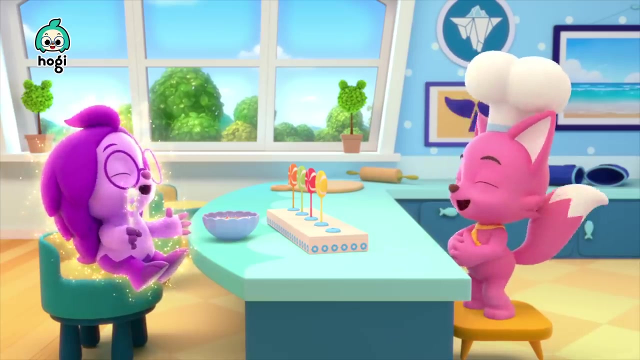 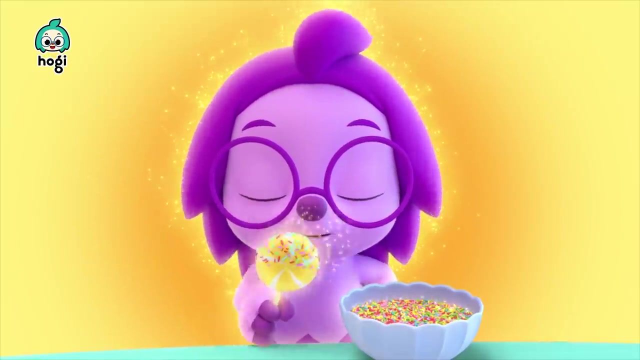 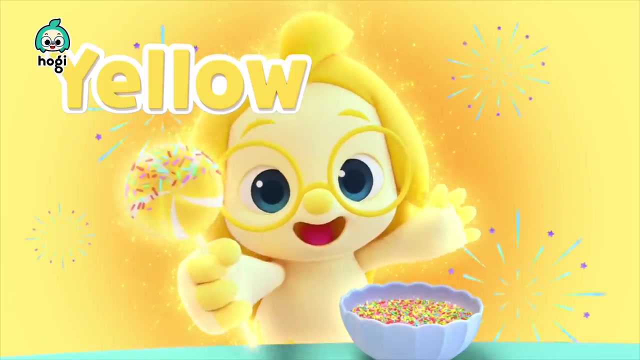 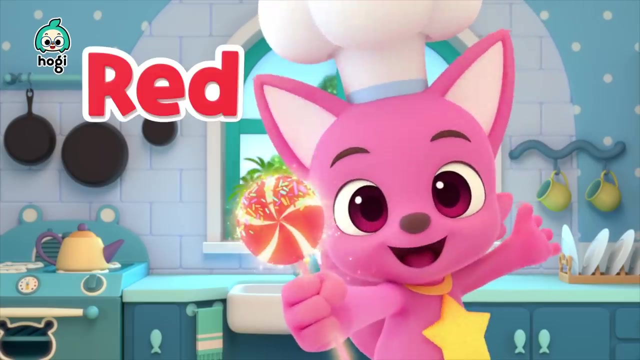 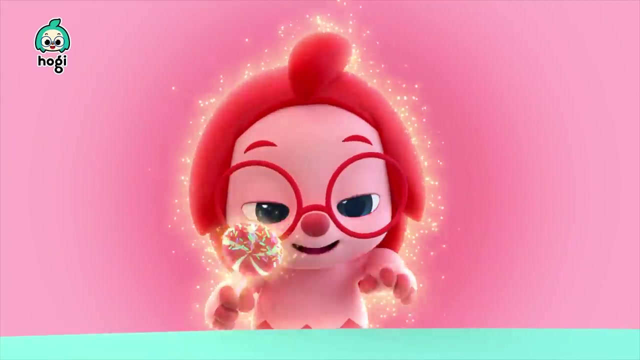 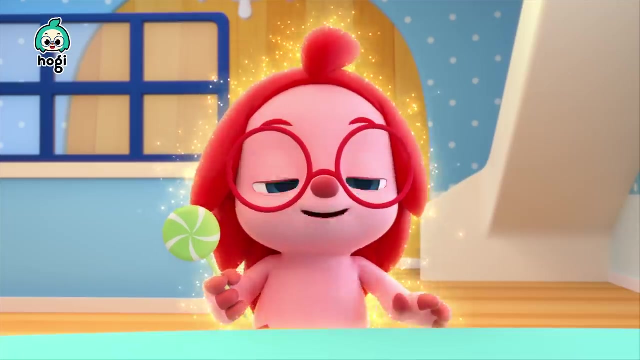 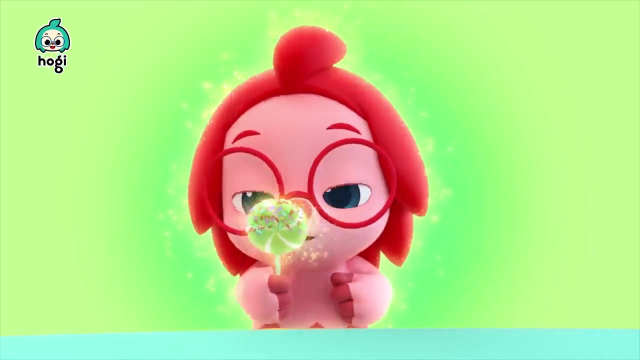 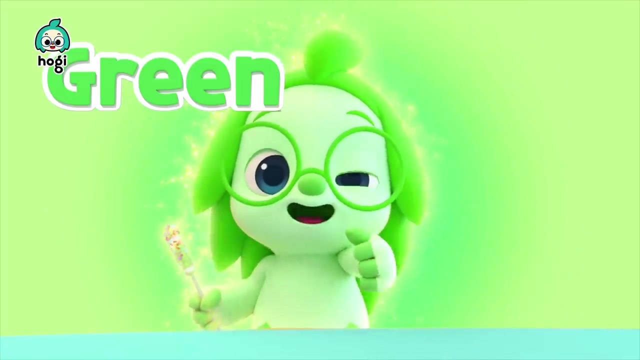 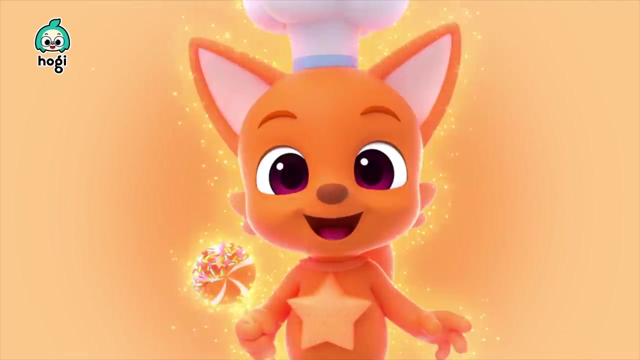 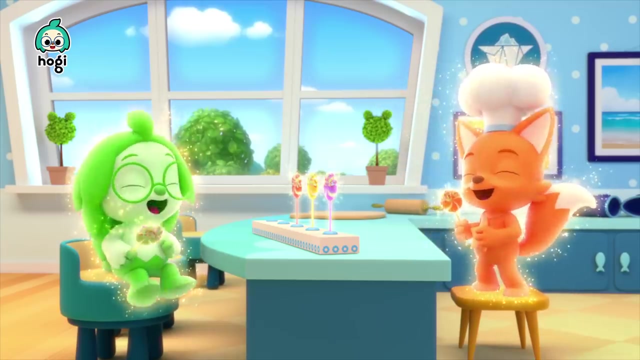 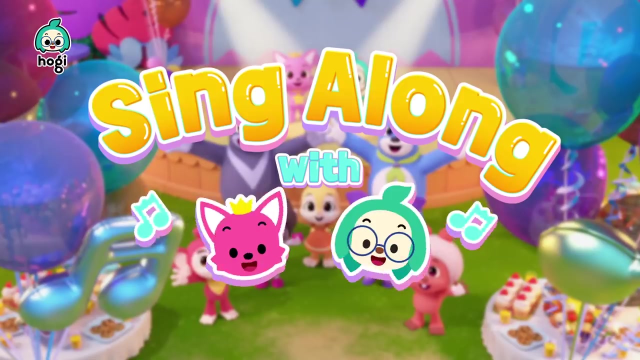 Hello, hello, Hoagie's friends. La-la-la-la-la-la Colors: Purple, Purple, Yellow, Yellow, Red, Red, Green, Green, Haha, Orange Sing along with Pinkfong and Hoagie. Thanks for the meal. 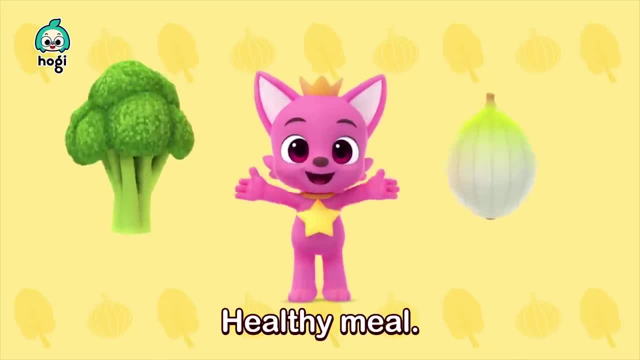 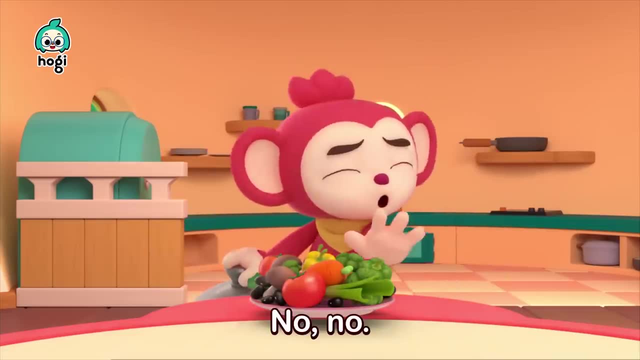 Yum yum yum, eat it too. Yum yum, yum. healthy meal. Yum yum yum, eat it too. Let's have a healthy meal. Yum, yum, Don't be picky, no, no. 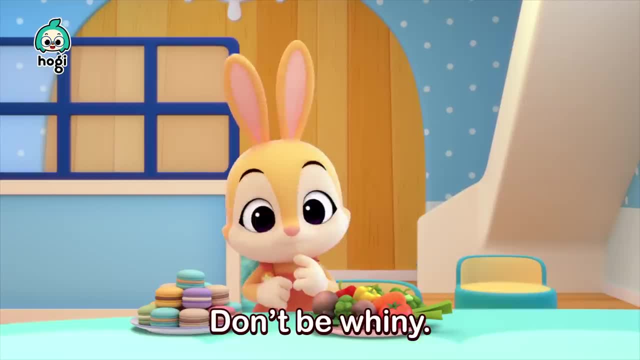 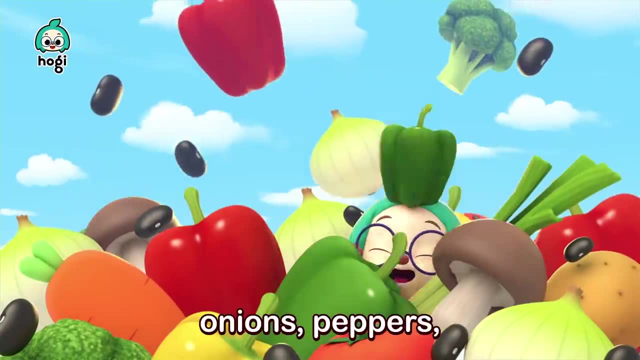 Let's have a healthy meal. Don't be whiny, no, no. Let's have a tasty meal: Broccoli, tomatoes, Onions, peppers and black beans. Have a seat and eat well. Let's have a healthy meal. 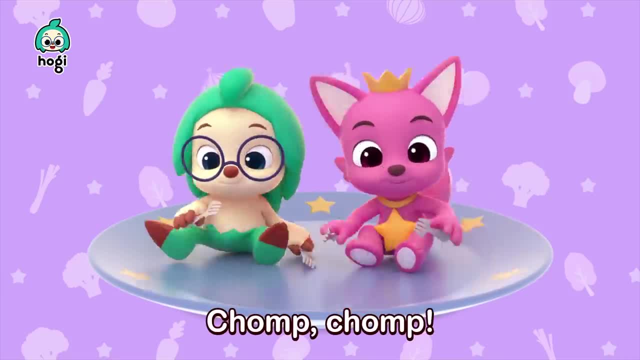 Okay, Chomp, chomp, chomp, chomp, chomp, chomp, chomp. Eat them all, Don't be picky. no, no, Let's have a healthy meal. Let's have a healthy meal. 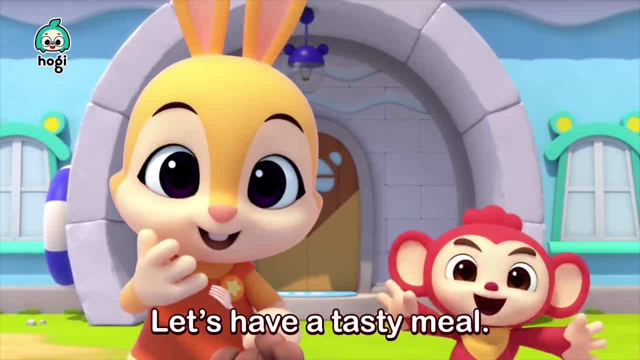 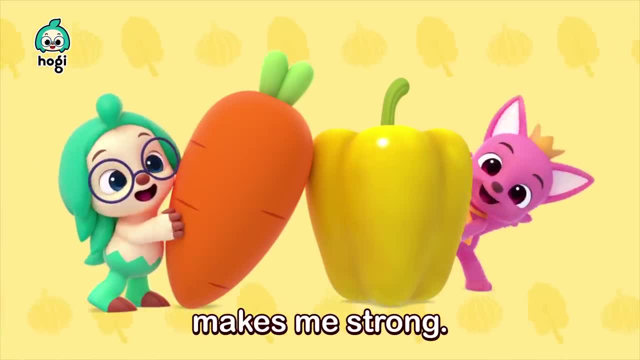 Don't be whiny, no, no, Let's have a tasty meal: Green spinach, potatoes, carrots, mushrooms and celery. Eating healthy makes me strong. Let's have a tasty meal. Okay, Yum yum, yum. eat it too. 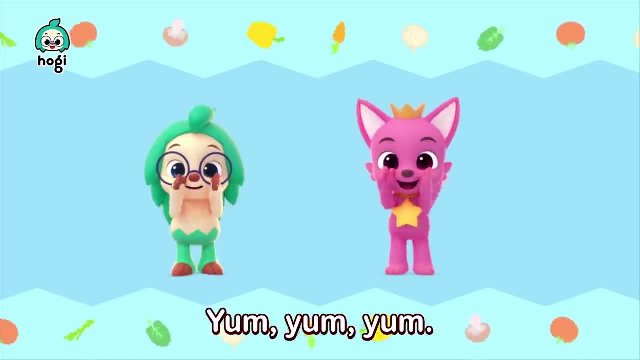 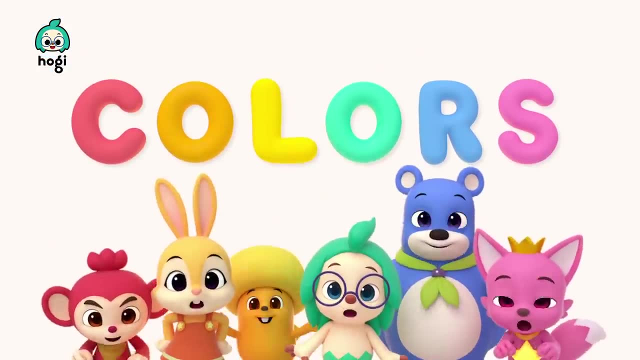 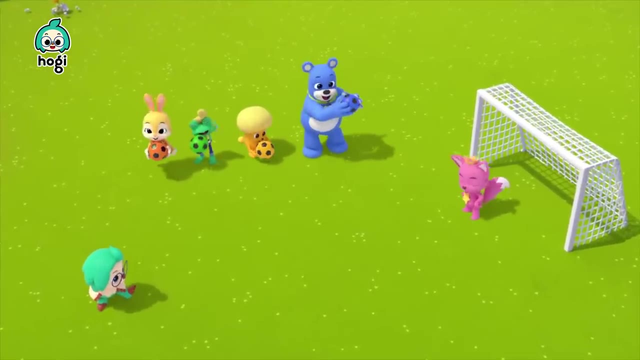 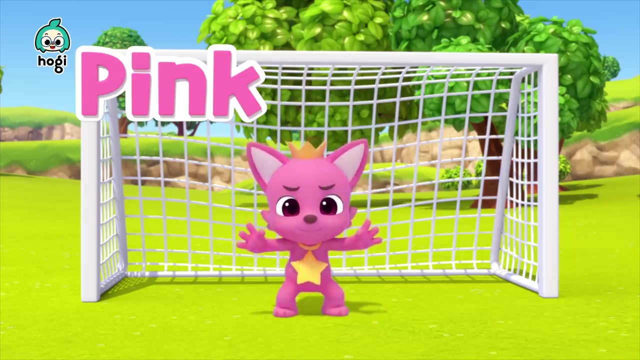 Yum yum yum healthy meal. Yum yum yum. eat it too. Let's have a healthy meal. Yum yum Colors Rumor home: Orange, Green, Yellow, Blue, Pink, Huh huh, huh. 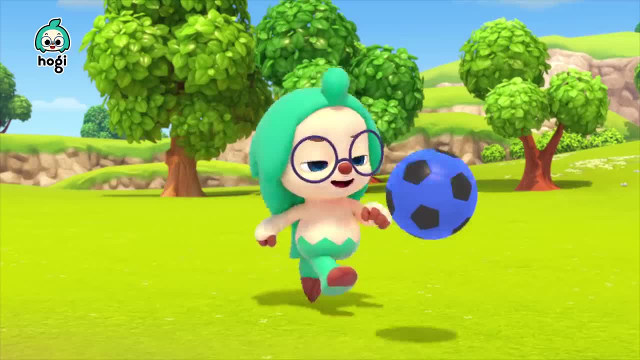 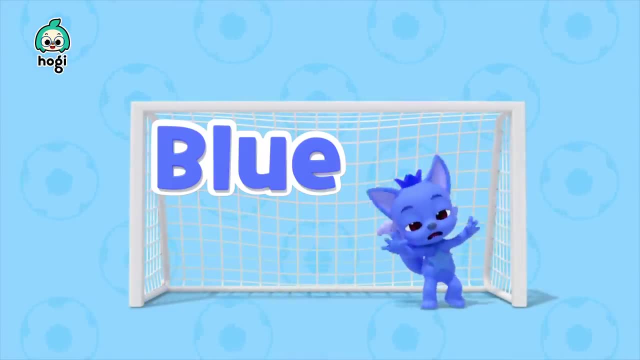 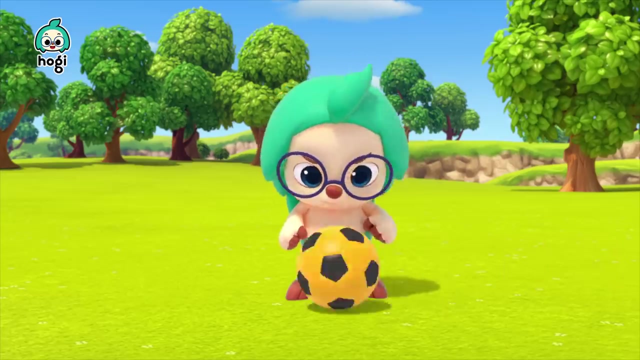 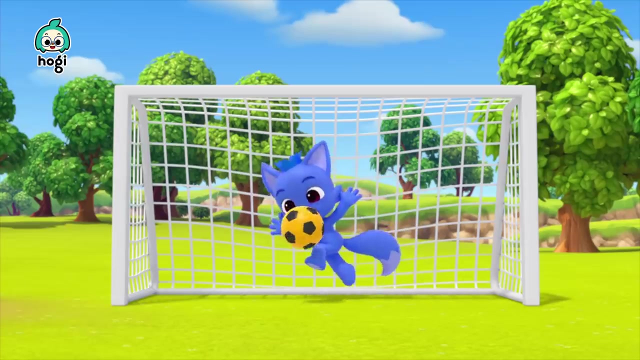 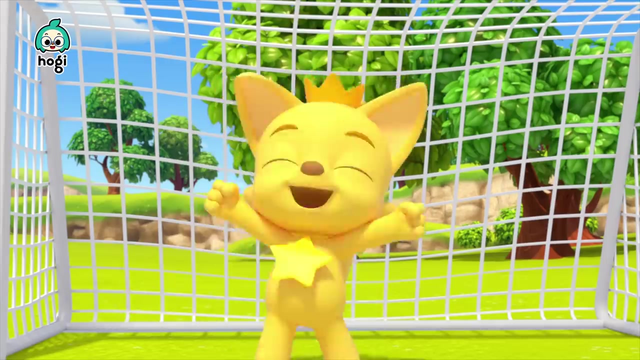 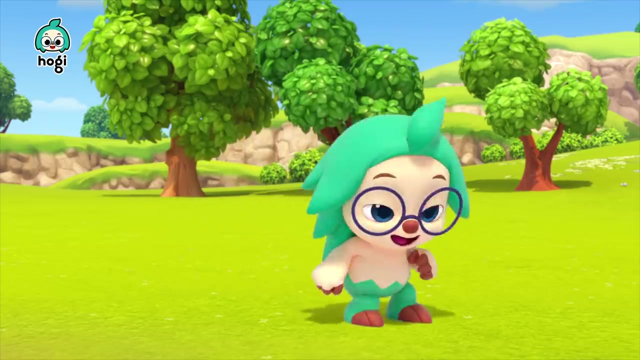 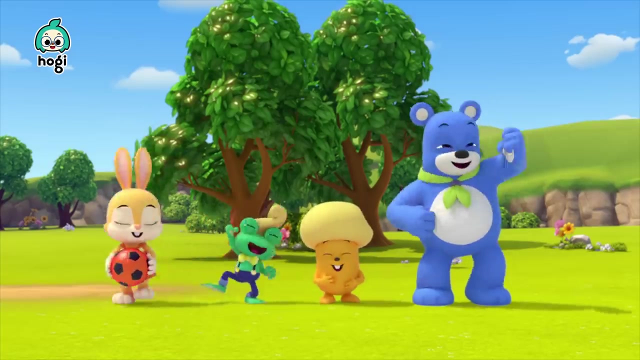 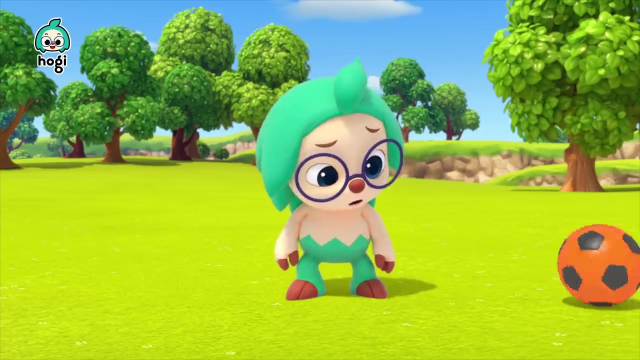 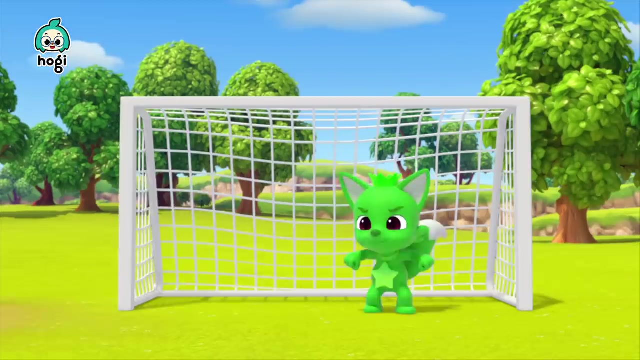 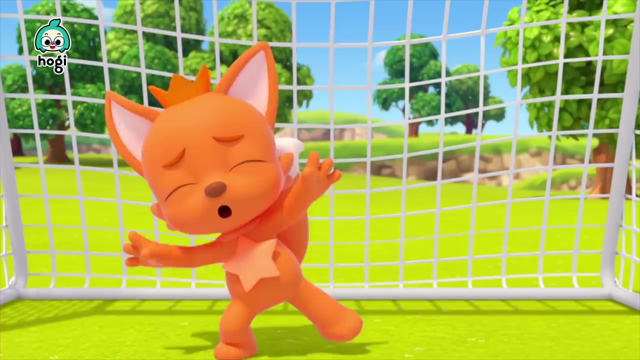 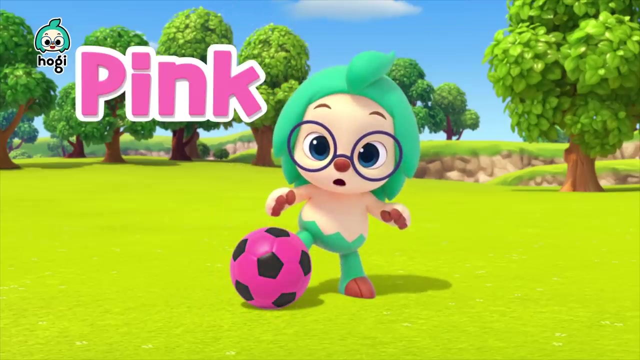 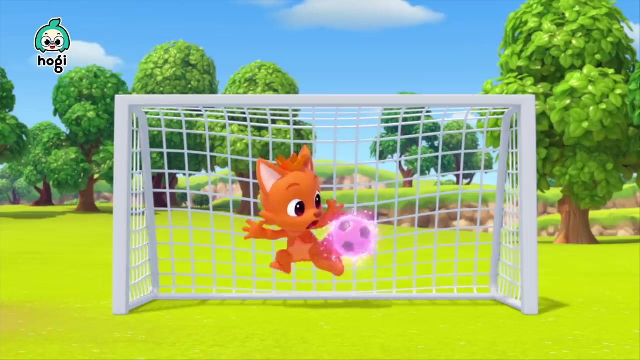 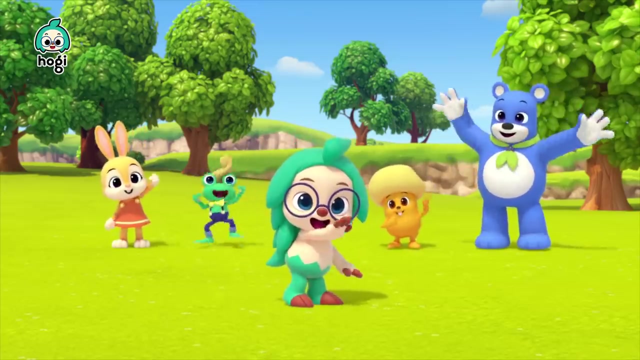 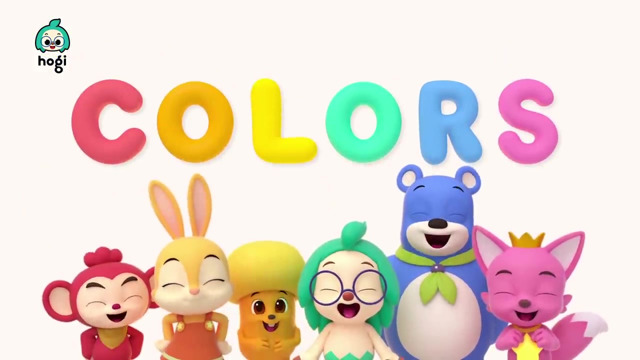 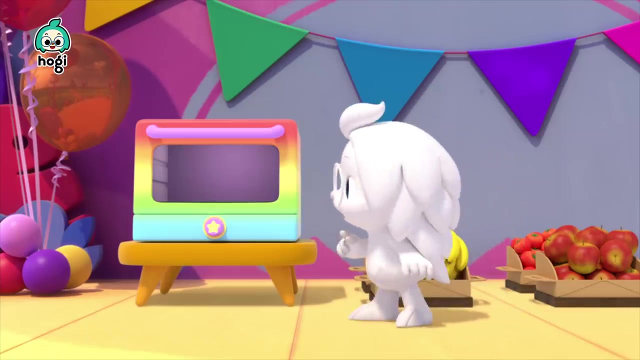 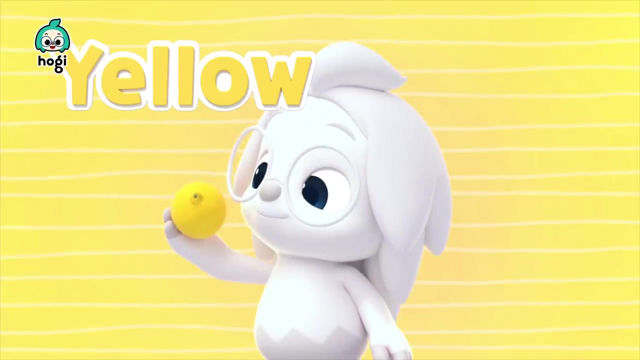 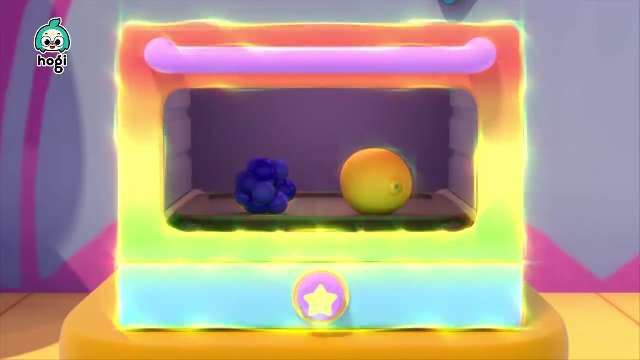 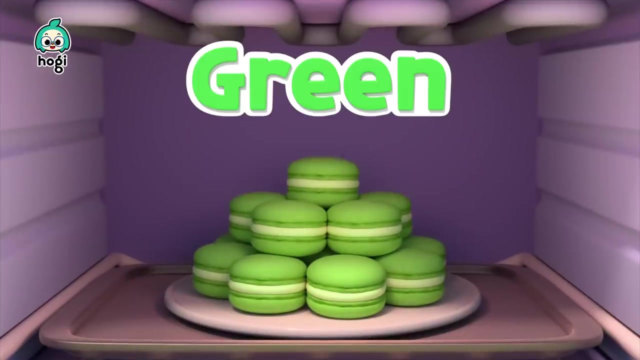 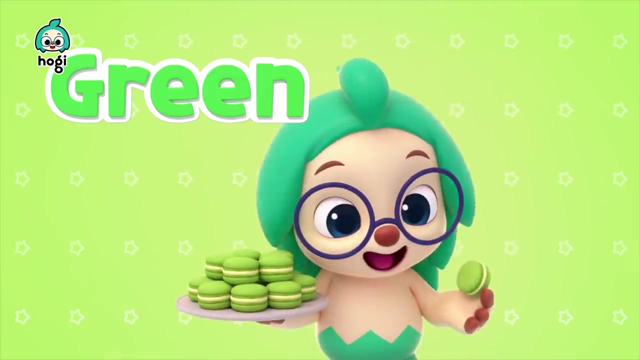 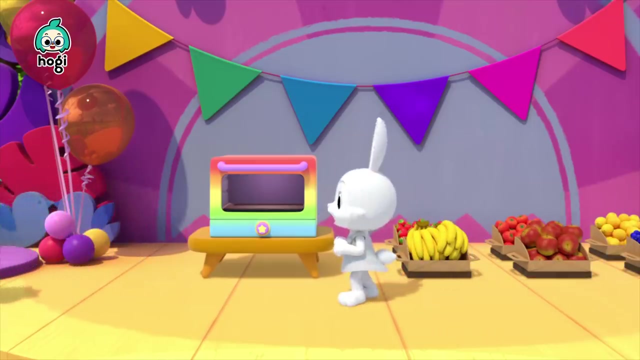 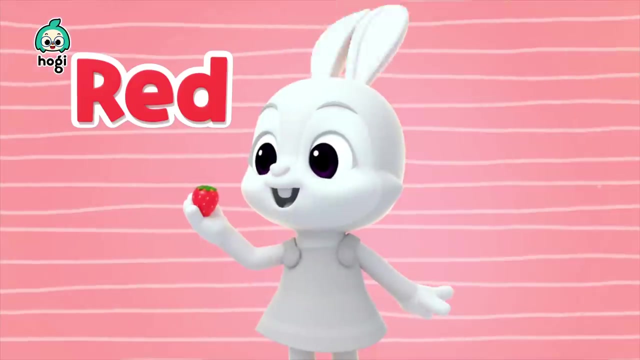 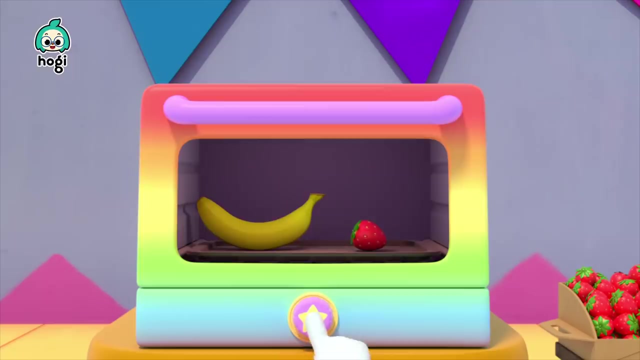 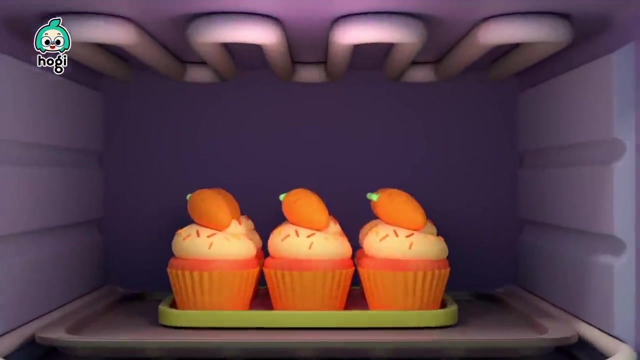 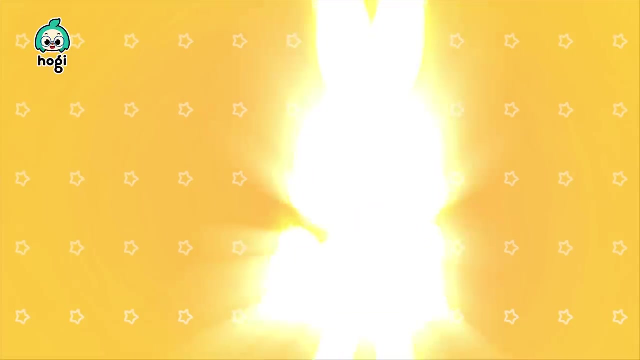 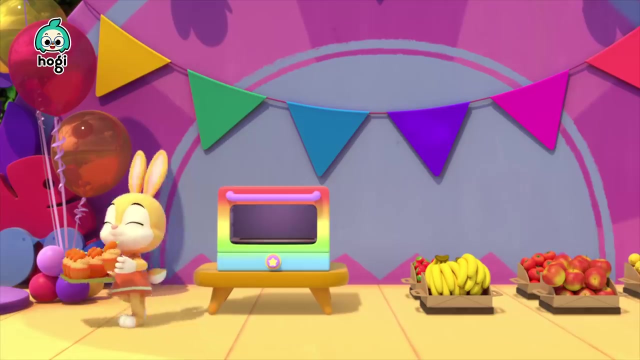 Blue, Blue, Yellow, Yellow, Green, Green, Green, Orange, Orange, Pink, Pink, Pink Colors: Yellow, Blue, Blue, Green, Green, Red, Yellow, Orange, Orange, Pink, Green, Yellow, White.